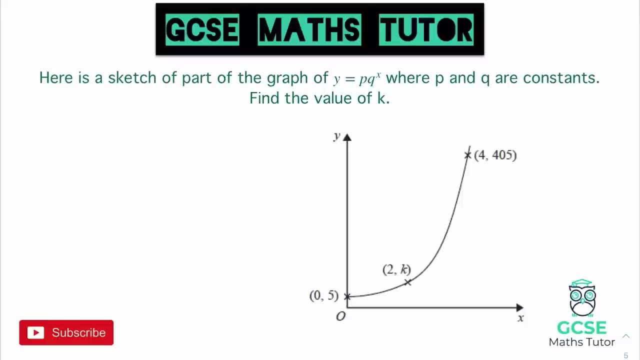 graphs that we're going to be applying throughout this video. Now, the question that's on the screen is the type of question that we're going to try and build up to, but we're going to start off with some of the more basic questions to start with and just build our way up to this one. 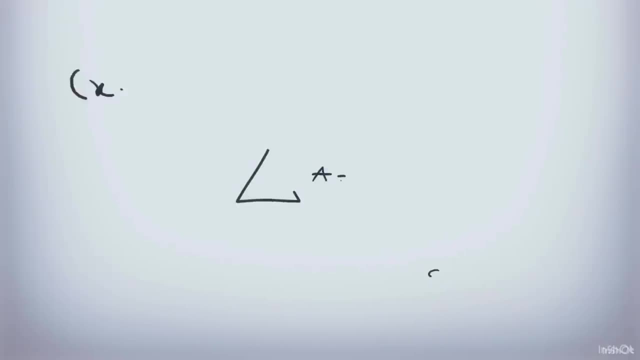 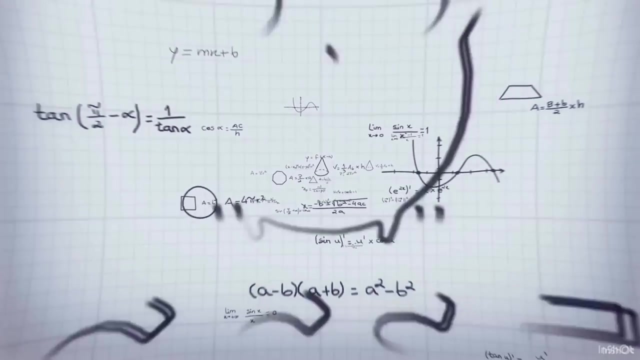 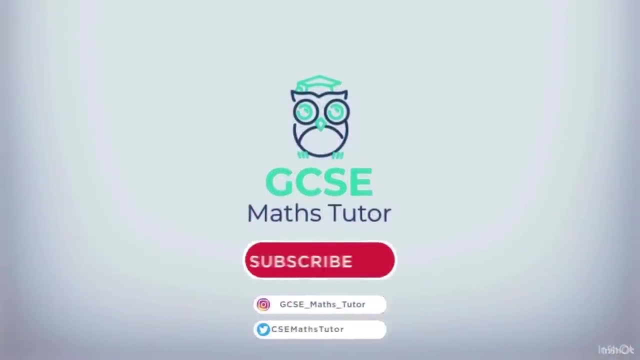 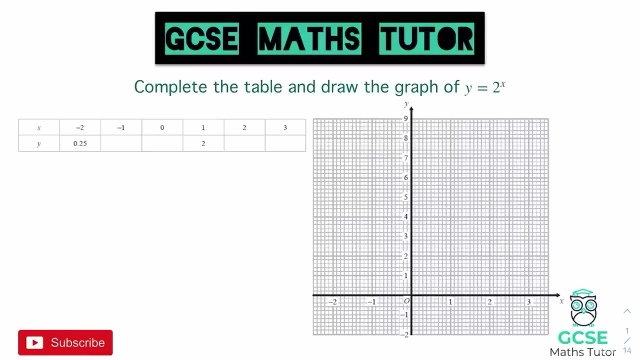 So, with that being said, let's get started. Okay, so the first question that we're going to have a look at is this one here, and it says: complete the table and draw the graph of y equals 2 to the power of x. and when we have this power of x, 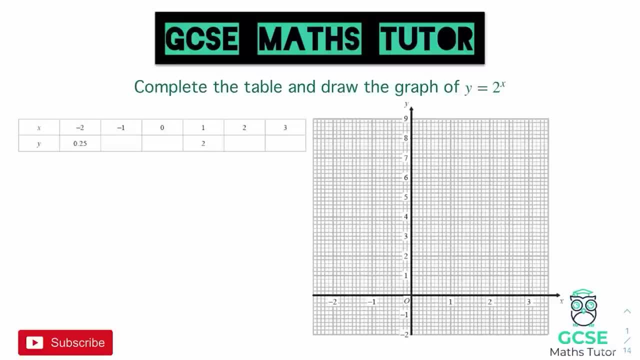 that's what defines our exponential graph when we have something linked to the power of our x value. Now this falls in very nicely with all the rest of coordinate geometry. Sometimes we're given a table, sometimes we're not. It does happen that with exponential 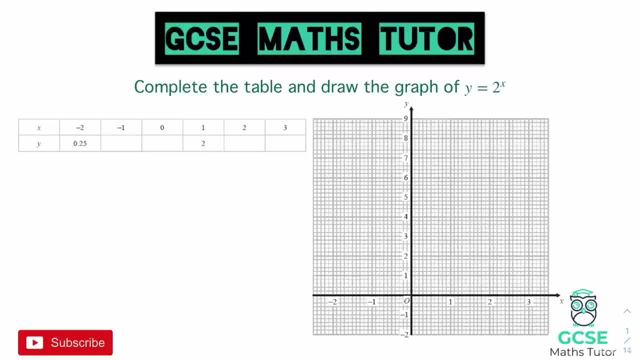 graphs, you're a little bit more likely to have a table than, say, with a straight line graph. but for the purpose of this one, we are going to have some tables included. Now, if we have a look at our table, we've got the values from negative 2 going up to 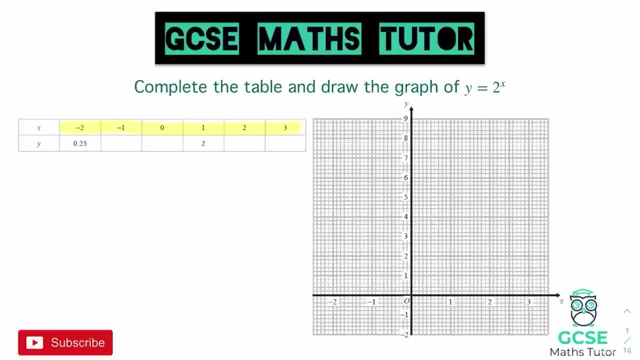 3 along our x values and, just like with normal coordinate geometry, all we have to do is plug that into the formula to find our y coordinate. Now remember, our little formula is at the top here, so it says that the y coordinate is equal to 2 to the power of the x coordinate. 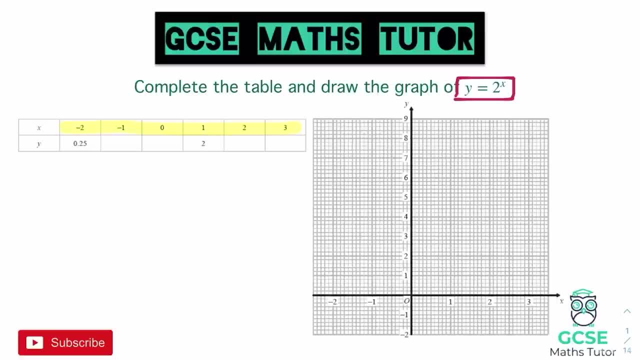 and that's what those y's and x's represent, obviously when we're looking at coordinate geometry. So to find our corresponding y value, we just need to figure out this one here. So, having a look- and it's always worth checking any that you have been given, so in this particular one here, 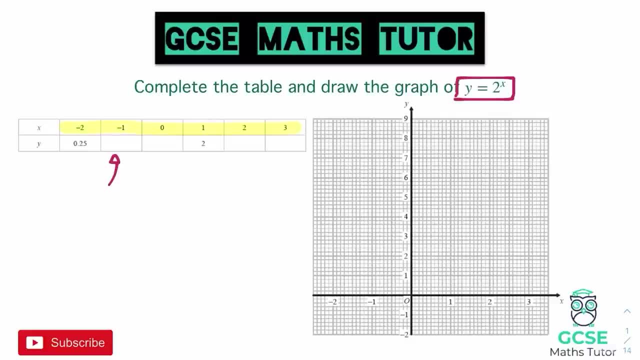 we've been given the y value for when x is negative, 2, and if I stick that into the calculator we get 2 to the power of negative 2.. Now if we put that in we get a quarter, which is 0.25. so just making 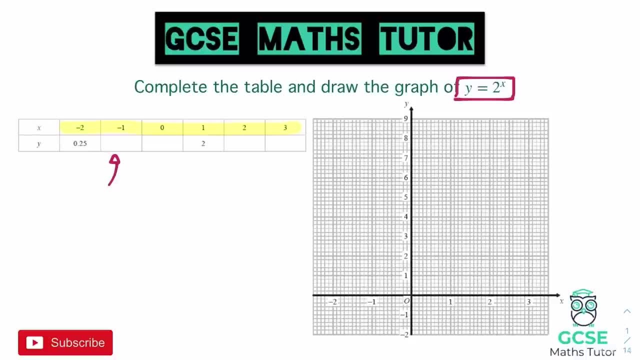 sure that, obviously, if you are using a calculator, you're getting the same answer that's given to you in the table. that's going to allow you to know that your methods are going to be correct for the other values there. But not forgetting- and here's where our first- 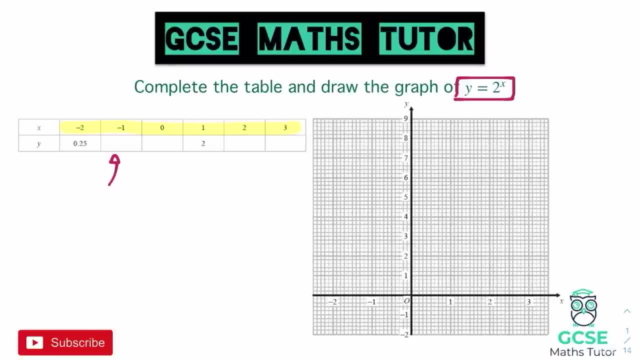 topic comes in, that if this was non-calculator we would have for this one 2 to the power of negative 1, and obviously that links into our fractional and negative indices, or in this case a negative indices, and I'll link the video to that in the description to make. 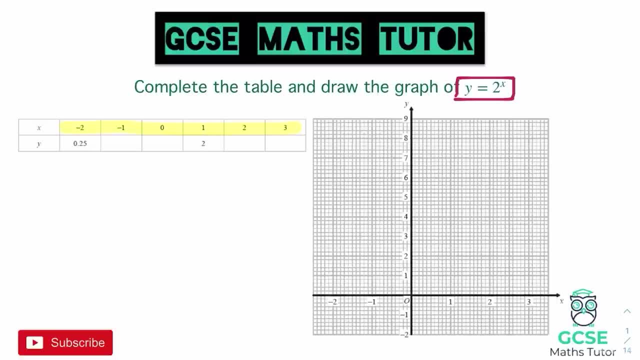 x coordinate. That's what those y's and x's represent, obviously, when we're looking at coordinate geometry. So to find our corresponding y value, we just need to figure out this one here. So, having a look- and it's always worth checking any that you have been given- So 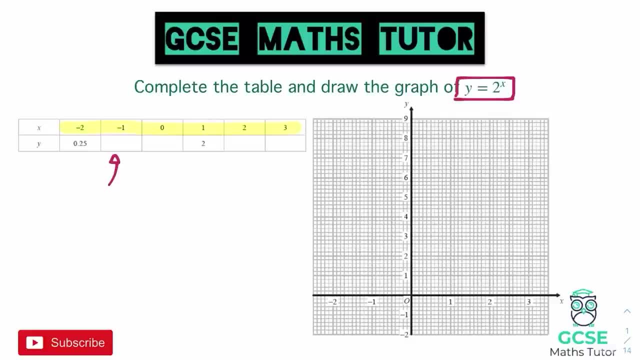 in this particular one. here we've been given the y value for when x is negative 2.. And if I stick that into the calculator we get 2 to the power of negative 2.. Now if we put that in we get a quarter, which is 0.25.. 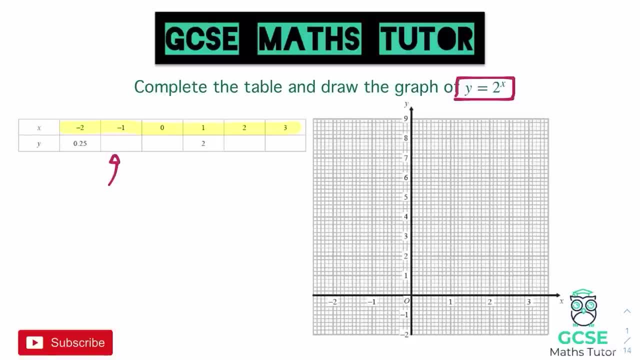 0.25.. 0.25., 0.25.. So just making sure that, obviously, if you are using a calculator, you're getting the same answer that's given to you in the table. That's going to allow you to know that your 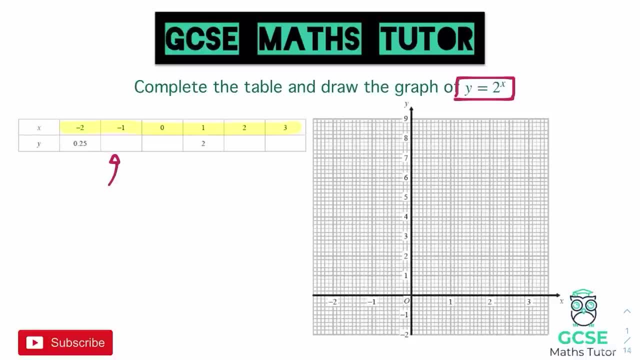 methods are going to be correct for the other values there. But not forgetting- and here's where our first topic comes in- that if this was non-calculator we would have for this one 2 to the power of negative 1.. And obviously that links into our fractional and negative. 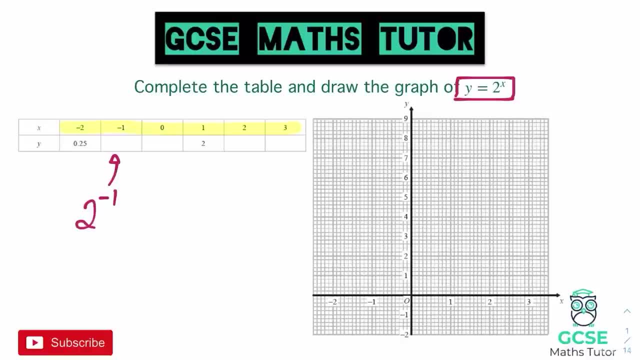 indices, or in this case, a negative indices, And I'll link the video to that in the description to make sure you can do this without a calculator as well. But I am going to be using a calculator throughout these questions. So the power of negative 1 just means that you flip it over, you do the reciprocal and 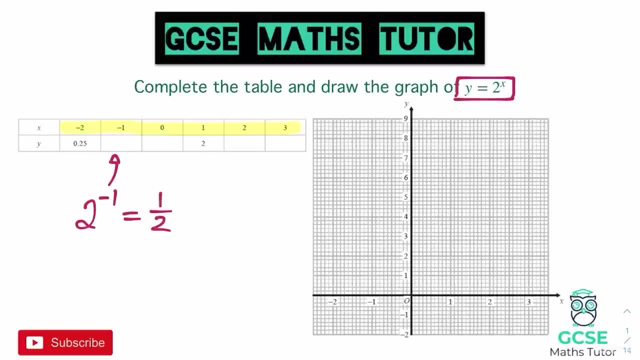 we have a power of 1, so that would become 1 over 2, or 0.5, and we can put that straight in 0.5.. The next one: here we've got 2 to the power of, and our x value this time is 0, so we've 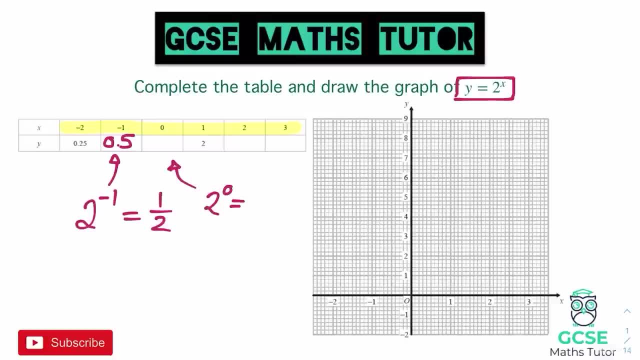 got 2 to the power of 0, and, remembering anything to the power of 0 is equal to 1, so our value there is 1.. That falls true for the next one. we've got 2 to the power of 1,, which is 2, and then 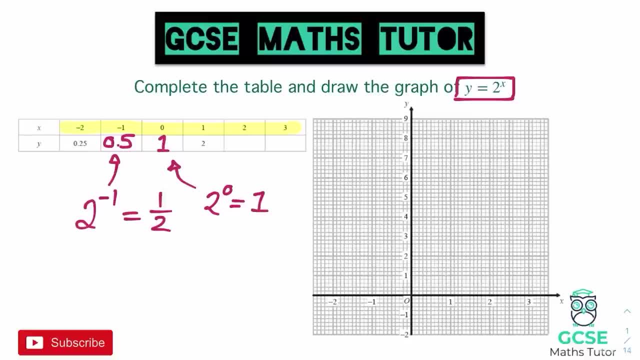 for the next 2 there, or the final 2,. we've got 2 to the power of 2, or 2 squared, which is 4, and then the final one. we have 2 to the power of 3, or 2 cubed, which is 8, and 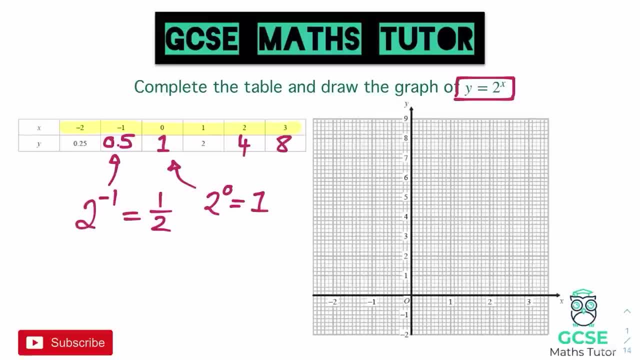 there we go. we have all our values. As I said, a lot of links here with normal coordinate geometry. I'll draw another graph, so we just need to plot these points So nice and carefully. negative 2 to 0.25, and that's a little bit fiddly for me to get. 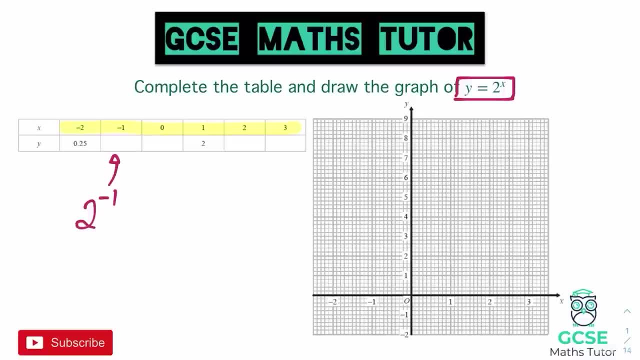 sure you can do this without a calculator as well, but I am going to be using a calculator throughout these questions. The power of negative 1 just means that you flip it over, you do the reciprocal and we have a power of 1, so that would become 1 over 2 or 0.5. we can put that straight in 0.5.. The next one: here we've. 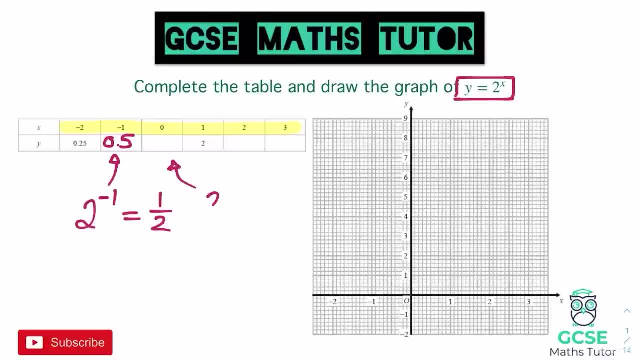 got 2 to the power of and our x value this time is 0. so we've got 2 to the power of 0 and remembering anything to the power of 0 is equal to 1, so our value there is 1.. That falls true for the next. 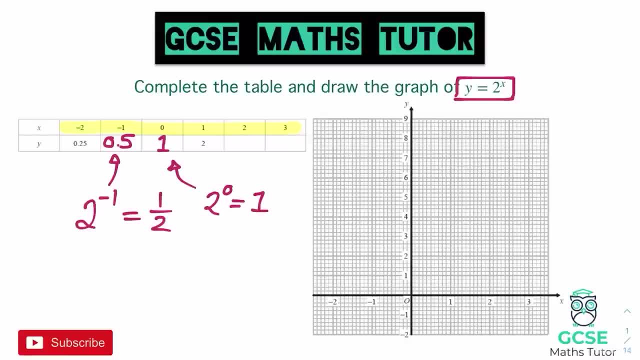 one: we've got 2 to the power of 1, which is 2, and then for the next 2 there or the final 2, we've got 2 to the power of 2, or 2 squared, which is 4, and then the final one: we have 2 to the power of 3 or 2. 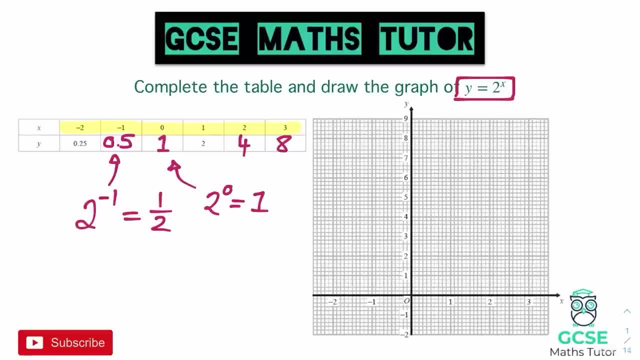 cubed, which is 8. and there we go. we have all our values. As I said, a lot of links here with normal coordinate geometry or drawing another graph, so we just need to plot these points So nice and carefully. negative 2 to 0.25. and that's a little bit fiddly for me to get to there, but I'm going. 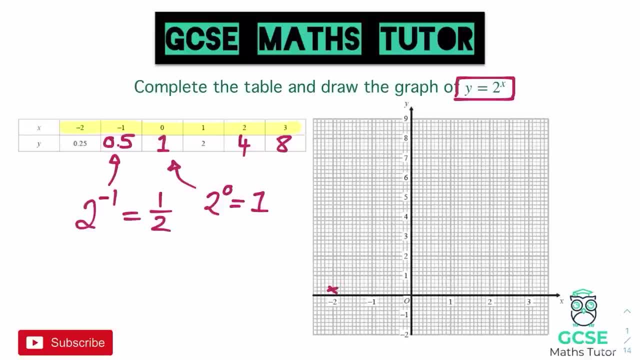 to try my best, there we go. so minus 2, 0.25, minus 1, we have 0.5,. 0, we have 1, we have 2,. 2 goes to 4 and then 3 goes up to 8, and that is, let me make sure I put it on the right. 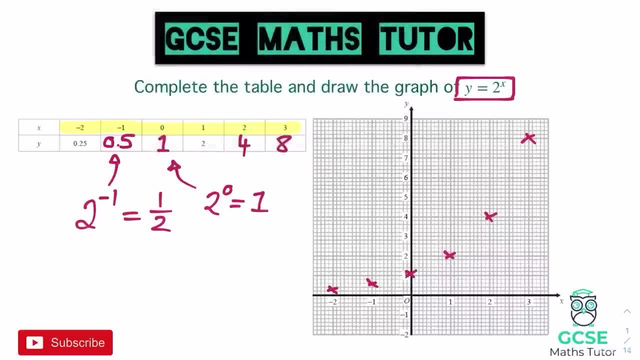 line just there. Now, when it comes to an exponential graph, we're going to draw a nice smooth curve, just like we do when we're drawing quadratics or cubics. so let's just draw a nice smooth curve, not with a straight line, not with a ruler, and there we go, just making sure that you join up all of those. 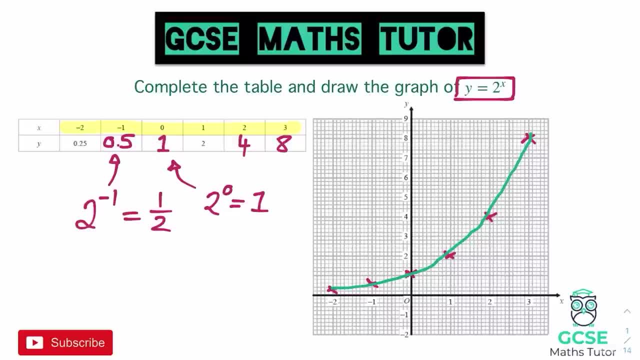 points as best you can. So there we go. there is our exponential graph. there's a few things that we're going to be looking at here. So if you're drawing exponential graphs, particularly with these simpler ones, you have a y intercept there of 1.. Now, thinking about the logic here, the x coordinate: 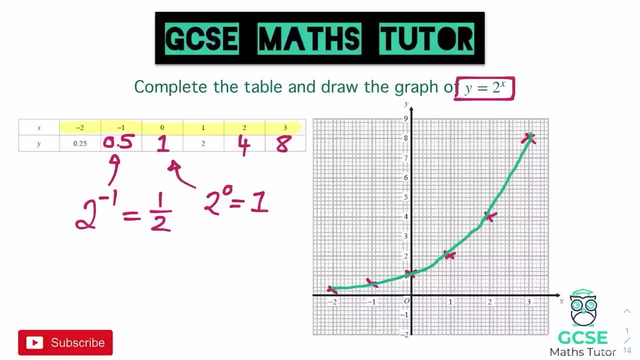 is 0 on that point, and anything to the power of 0 is 1, so any exponential graph that's given to us in this way, something to the power of x, is always going to cross through the point 1 on the y axes. Okay, so, something really important to remember. obviously, with these exponential graphs, which 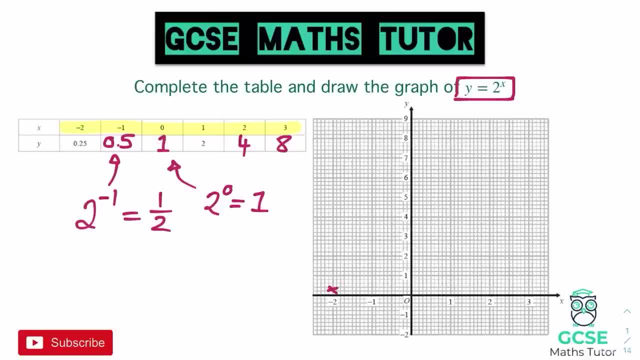 to there, but I'm going to try my best. there we go. so, minus 2, 0.25, minus 1, we have 0.5, 0.5.. 0, we have 1, 1, we have 2, 2 goes to 4, and then 3 goes up to 8, and that is, let me make. 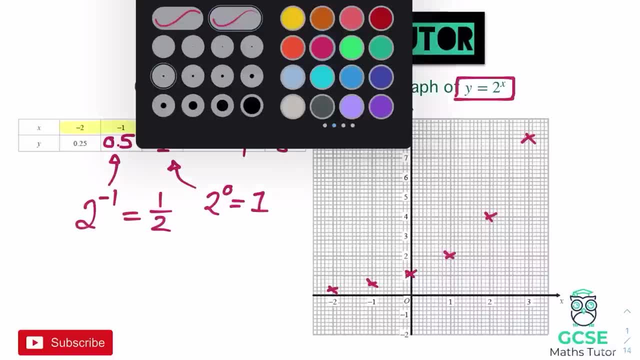 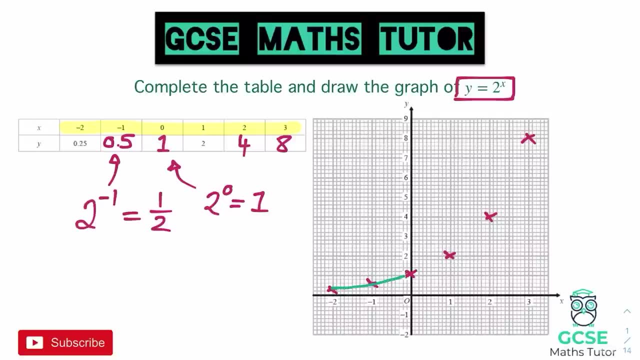 sure I put it on the right line just there. Now, when it comes to an exponential graph, we're going to draw a nice smooth curve, just like we do when we're drawing quadratics or cubics. So let's just draw a nice smooth curve, not with a straight line, not with a ruler, and 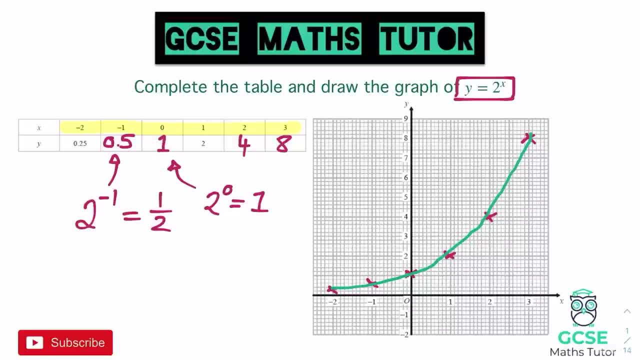 there we go, just making sure that you join up all of those points as best you can. So there we go. there is our exponential graph. There's a few things that you'll notice about these exponential graphs, particularly with these simpler ones. 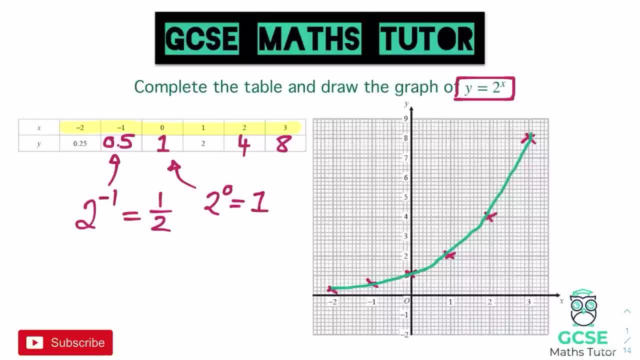 You have a y intercept there of 1.. Now, thinking about the logic here, the x coordinate is 0 on that point, and anything to the power of 0 is 1, so any exponential graph that's given to us in this way, something to the 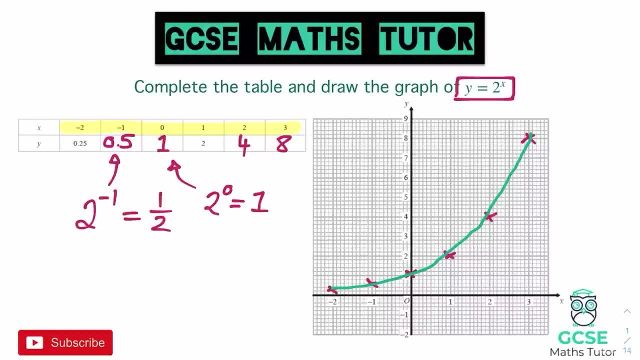 power of x is always going to cross through the point 1 on the y axis. Okay, so something really important to remember, obviously with these exponential graphs which you'll see on the next question, particularly if we're going to draw a sketch, it's just. 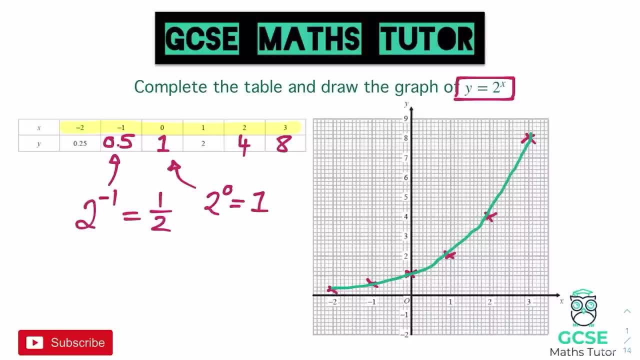 a nice, easy point to remember with these exponential graphs. Obviously, that would change were we to make this a bit more of a complex version of an exponential graph, but for the majority of them, they are going to pass through 1.. Right, let's have a look at our next question. 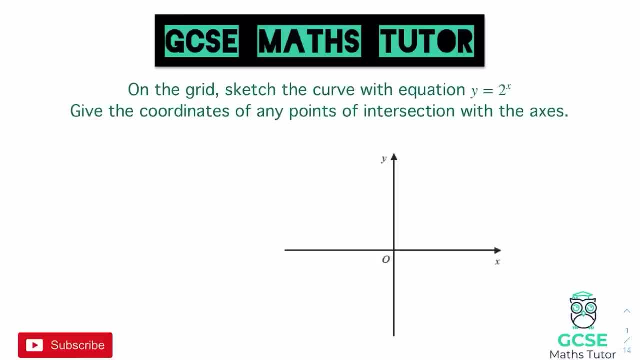 Okay, so this question is very closely linked to our first one and it's going to bring up some of the points that I was talking about just then. It says on the grid: sketch the curve with equation: y equals 2 to the power of x. so 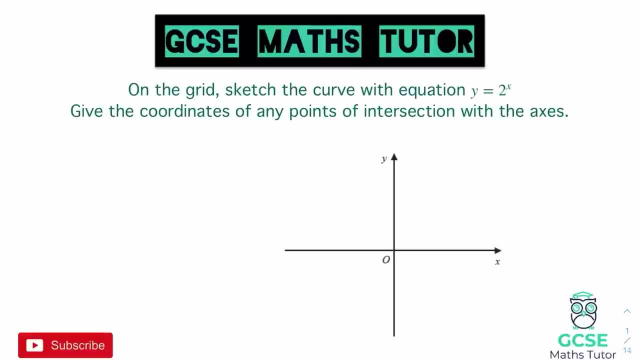 exactly the same one that we've just drawn. It says: give the coordinates of any points of intersection with the axis. Now, as we saw that exponential curve, it started over here in the negative region. it went across and then it started sloping upwards faster and faster, and that's what. 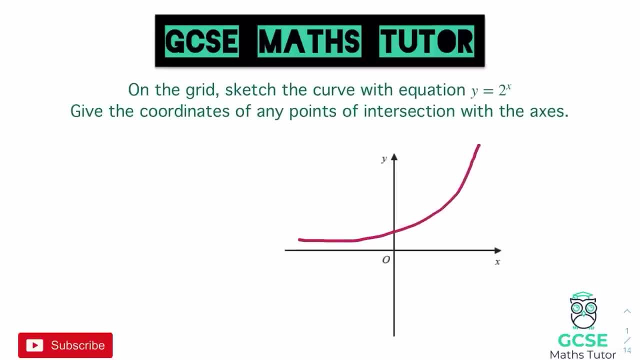 every exponential curve is going to look like, whether it's 3 to the power of x, 4 to the power of x, 5 to the power of x, they're all going to basically look exactly the same here. Obviously, if we were to draw them to scale and not as a sketch, you would see this emphasis. 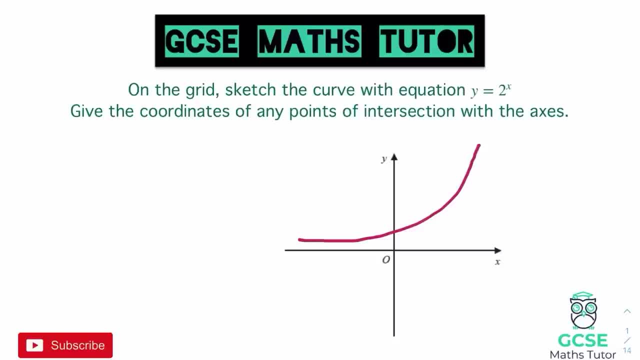 getting higher and higher on that part of the curve on the positive section. but in terms of a sketch they're all going to look just like this And we've already mentioned that it crosses through the y-axes. now again, it doesn't. 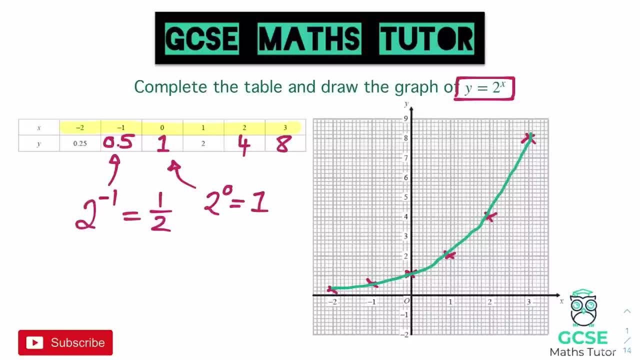 you'll see on the next question. Now I'm going to show you an example of an easy point to remember with these exponential graphs. Obviously, that would change were we to make this a bit more of a complex version of an exponential graph, but for the majority of them, they are going to pass through 1.. Right, let's have a look at our. 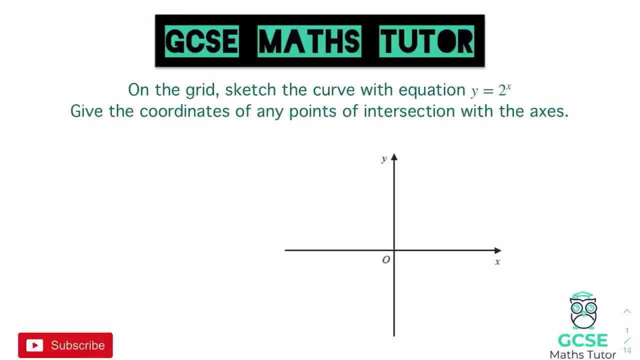 next question. Okay, so this question is very closely linked to our first one. it's going to bring up some of the points that I was talking about just then. It says on the grid: sketch the curve with equation y equals 2 to the power of x. so exactly the same one that we've just drawn. 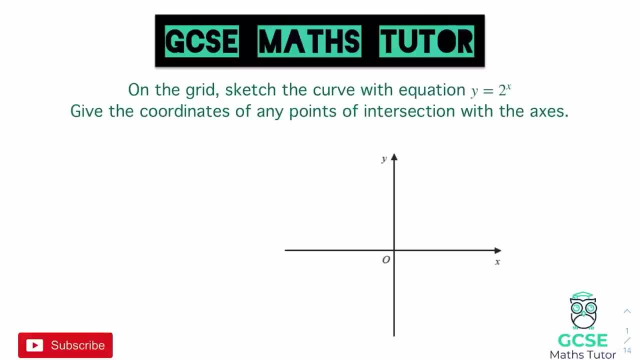 It says: give the coordinates of any points of intersection with the axes. Now, as we saw that curve, it started over here in the negative region, it went across and then it started sloping upwards faster and faster. and that's what every exponential curve is going to look like, whether it's 3 to the. 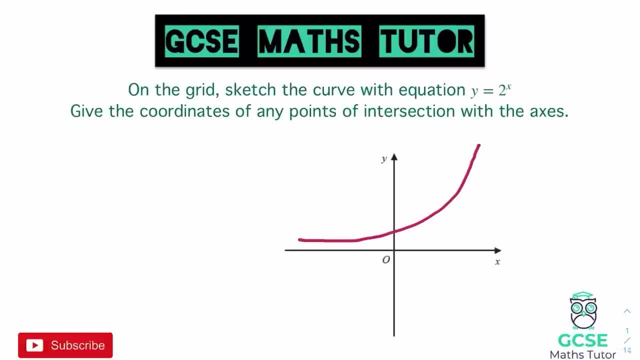 power of x, 4 to the power of x, 5 to the power of x. they're all going to basically look exactly the same here. Obviously, if we were to draw them to scale and not as a sketch, you would see this emphasis getting higher and higher on that part of part of the curve, on the positive section, but in 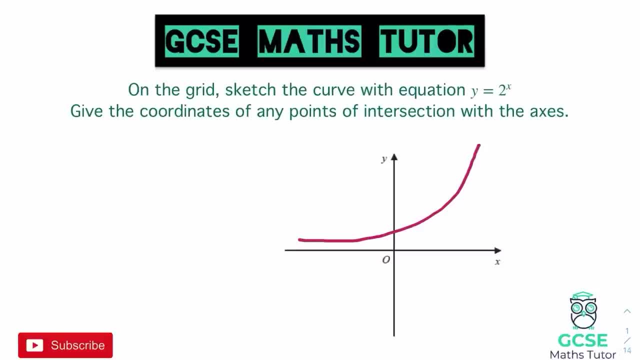 terms of a sketch. they're all going to look just like this one, and we've already mentioned that it crosses through the y-axis. Now again, it doesn't matter if it was 3 to the power of x, 4 to the power of x or anything. 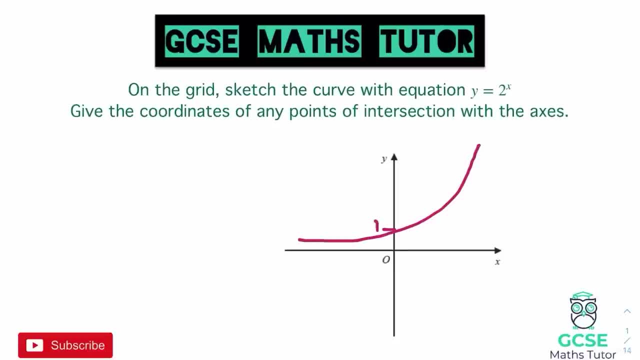 that is going to go through the y-intercept at 1.. And there we go. that's all we need to do for a sketch. So what you're going to have a little practice at is just making sure that you can fill in those tables and just making sure you're happy to draw a couple of these sketches to start. 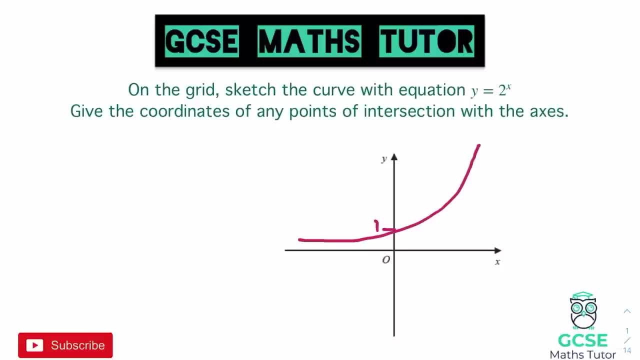 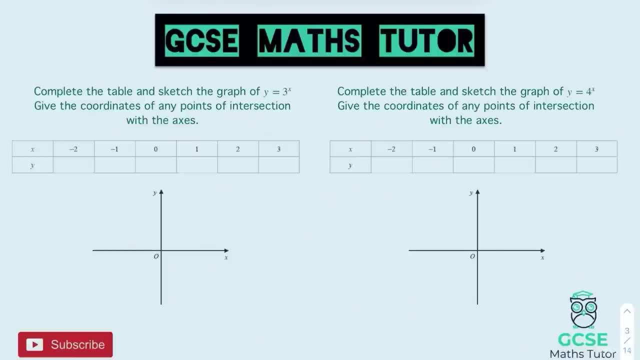 with, and then we'll have a look at some of these harder questions. So here we go, let's have a look at some for you to have a go at. Okay, so there's two questions on the screen for you to have a go at Now. what I want you to do with these is I want you to fill in the tables. We have two equations. 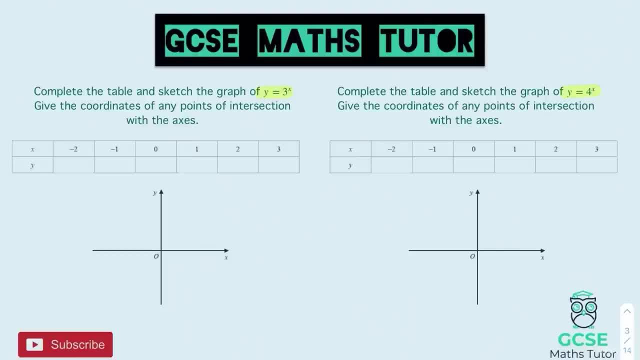 here, we've got y equals 3 to the power of x and we've got y equals 4 to the power of x. Again, you can use a calculator, but if you want to challenge yourself, you can do it without, and all I want you to do is draw a little sketch, very similar to mine again, showing where it crosses through the y-axis. 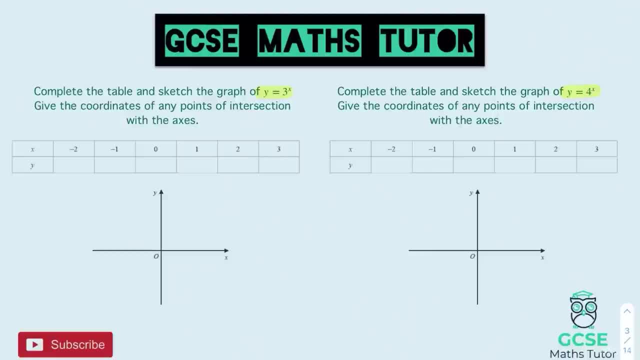 So there we go. there's your two questions. pause the video there and we'll have the answer in a sec. Okay, so moving on to this first question, we've got 3 to the power of negative 2- and, as I said, you could use a calculator here- and 3 to the power of negative 2 is 1 over 9, which isn't the nicest. 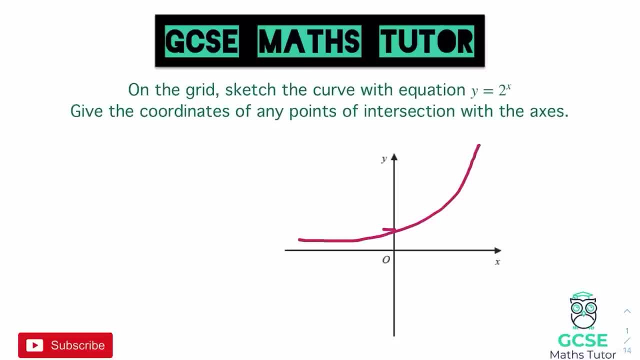 matter if it was 3 to the power of x, 4 to the power of x or anything that is going to go through the y-intercept at 1.. And there we go. that's all we need to do for a sketch. 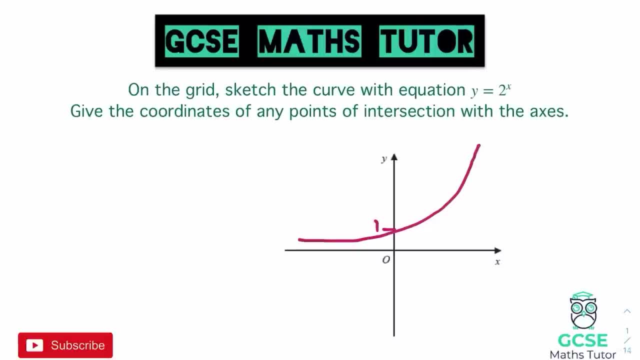 So what you're going to have a little practice at is just making sure that you can fill in those tables and just making sure you're happy to draw a couple of these sketches to start with, and then we will have a look at some of these harder questions. 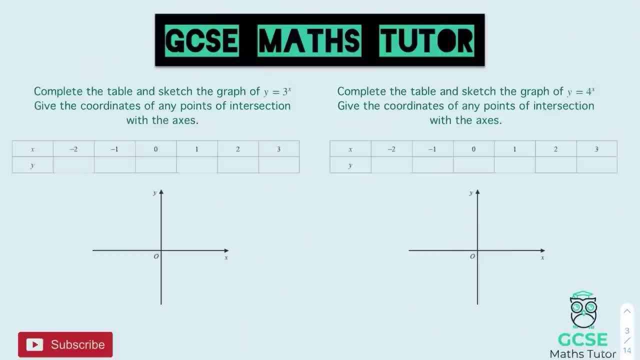 So here we go, let's have a look at some for you to have a go at. Okay, so there's two questions on the screen for you to have a go at Now. what I want you to do with these is I want you to fill in these. 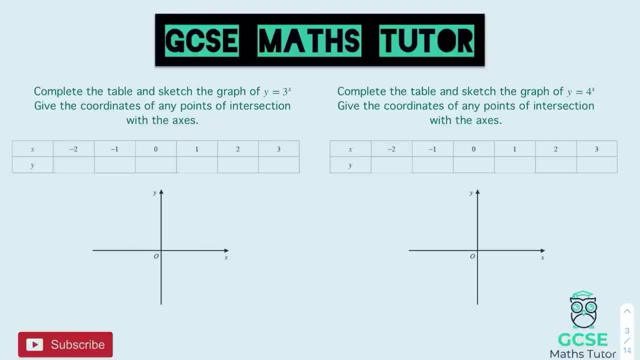 Okay, The tables. we have two equations here. we've got y equals 3 to the power of x and we've got y equals 4 to the power of x. Again, you can use a calculator, but if you want to challenge yourself, you can do it. 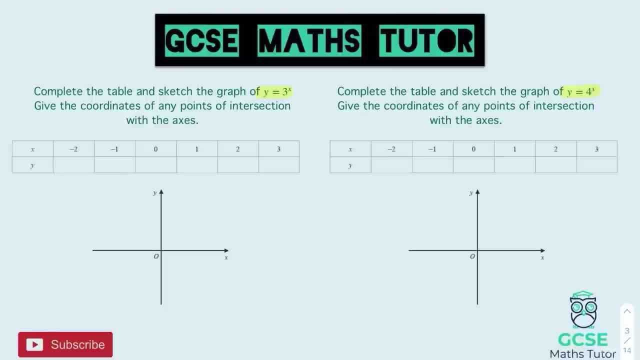 without, And all I want you to do is draw a little sketch, very similar to mine again, showing where it crosses through the y-axes. So there we go. there's your two questions. pause the video there and we'll go over the. 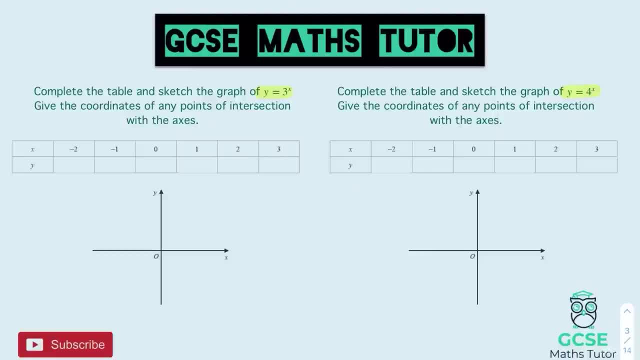 answer in a sec. Okay, so moving on to this first question, we've got 3 to the power of negative 2, and, as I said, you could use a calculator here- and 3 to the power of negative 2 is 1 over. 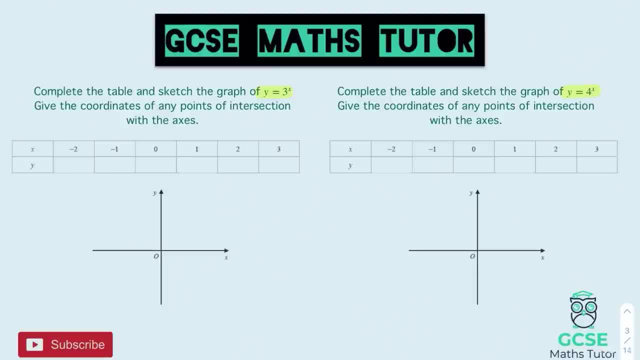 9,, which isn't the nicest there, and it doesn't matter whether you put that in as a recurring decimal or whether you write it in as a fraction. I'm just going to write it in as 1. 9th Onto the next one, we've got 3 to the power of negative 1, which is 1. 3rd again, you could. 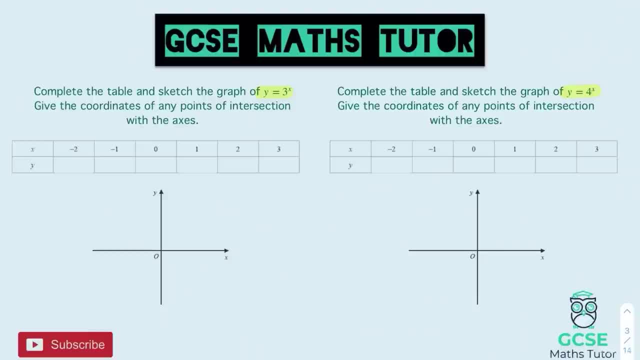 there, and it doesn't matter whether you put that in as a recurring decimal or whether you write it as a fraction. I'm just going to write it in as 1, 9th Onto the next one. we've got 3 to the power. 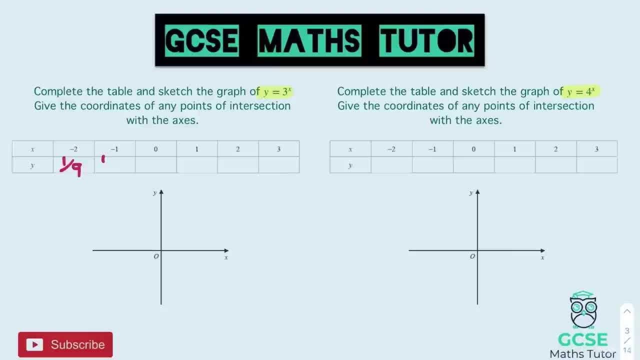 of negative 1, which is 1. 3rd, Again, you could write that as 0.3 recurring. I'm just going to leave them as fractions. 0. anything to the power of 0 is 1. then we have 3 to the power of 1,. 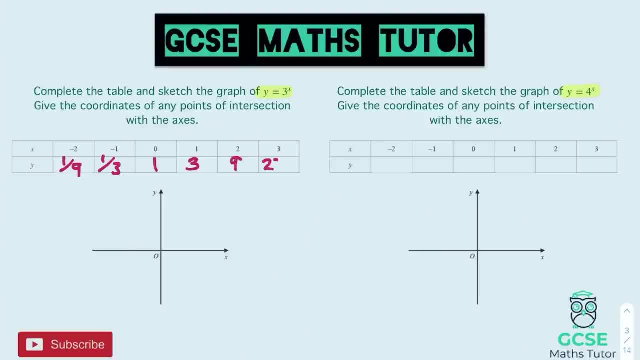 3 squared for 9, and 3 to the power of 3, which is 27.. And again, just drawing a little sketch, as long as it's sloping up in that positive direction and we have the y intercept of 1.. Okay, so moving on to our next one. So for this second one, here we've got 4 to the power of 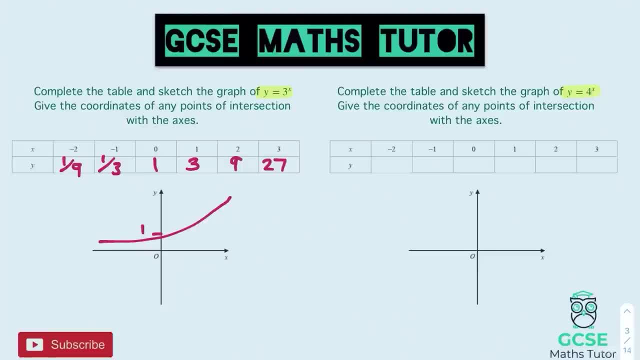 negative 2.. So 4 to the power of negative 2 is 1 over 16.. 4 to the power of negative: 1 is 1 over 4.. 4 to the power of 0 is 1.. 4 to the power of 1 is 4.. 4 squared is 16 and 4 to the power of 3. 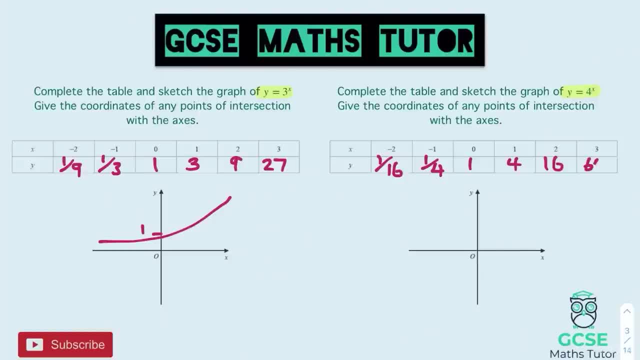 is 4. well, 16 times 4 again, which is 64.. And again, drawing a sketch, you could emphasize the fact that it's going to be sloping up more, but again, just emphasizing it crosses through the y-axis at 1.. So, as you can see, it's a little bit strange because both my sketches look pretty. 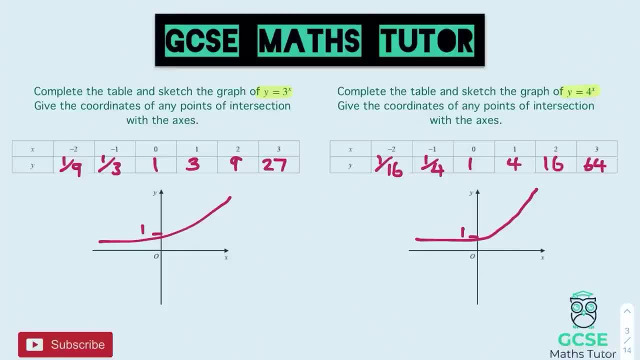 much the same. but again, we're not drawing it to scale, we're just showing the direction that it's sloping in and also the fact that it crosses the y-axis at 1.. So there we go again. obviously, you could have done that ever so slightly differently, because you could have put decimals in instead. 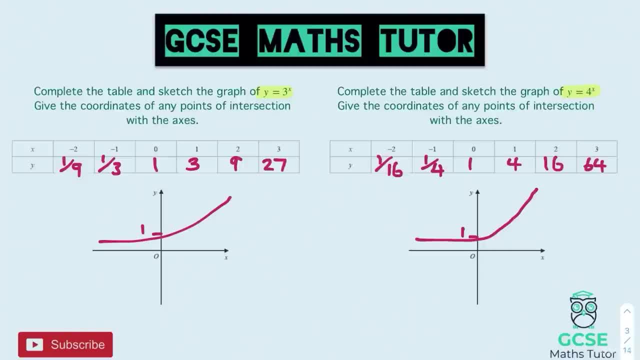 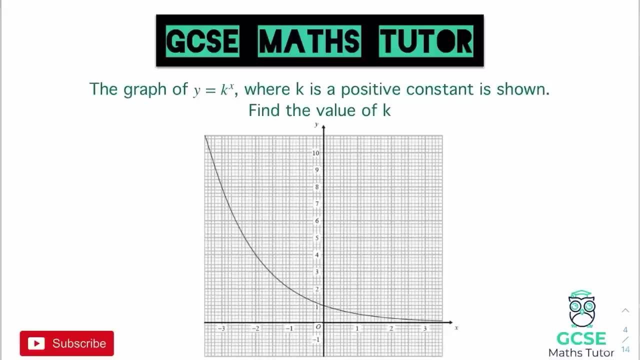 but obviously that's fine. you should be able to match up your decimals with my fractions there, Right? so let's have a look at a slightly trickier question. Here we've got a slightly different question. This is: the graph of y equals k to the power of x. 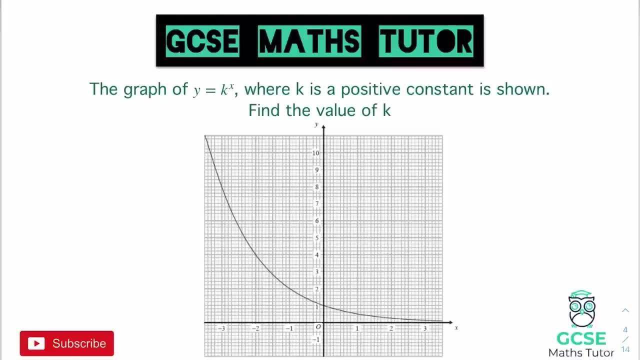 where k is a positive constant is shown. find the value of k. Now, that word constant just means that it is not necessarily a whole number. it could be a fraction as well. So when we're having a look at this, we just need to figure out how we're going to approach it. So we know it's going to be y equals. 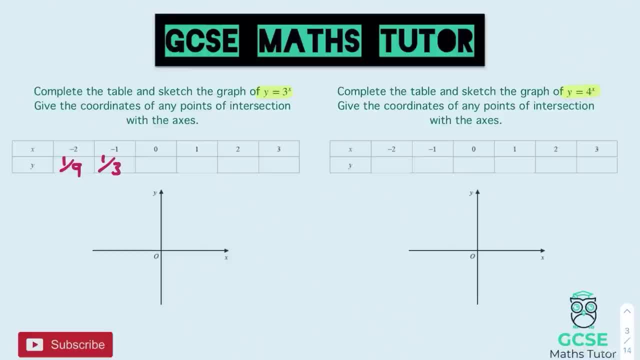 have write that as 0.3 recurring. I'm just going to leave them as fractions. 0, anything to the power of 0 is 1, then we have 3 to the power of 1, 3 squared for 9,. 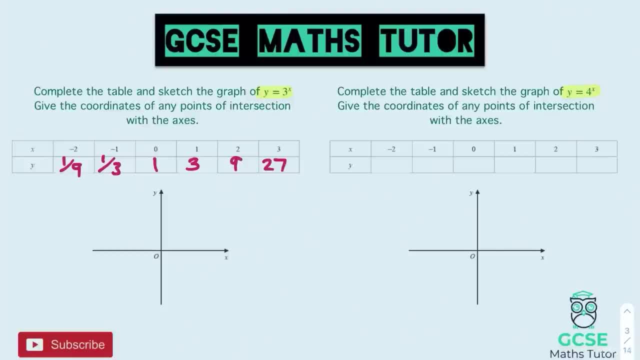 and 3 to the power of 3, which is 27.. And again, just draw in a little sketch, as long as it's sloping up in that positive direction and we have the y intercept of 1.. Okay, so, moving on to our next one. 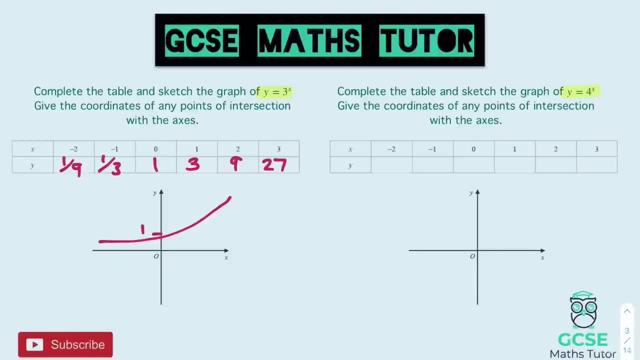 So for this second one here we've got 4 to the power of negative 2.. So 4 to the power of negative, 2 is 1 over 16,, 4 to the power of negative, 1 is 1 over 4,, 4 to the power of 0 is 1,, 4 to the power of 1 is 4,, 4 squared is 16, and 4 to the power. 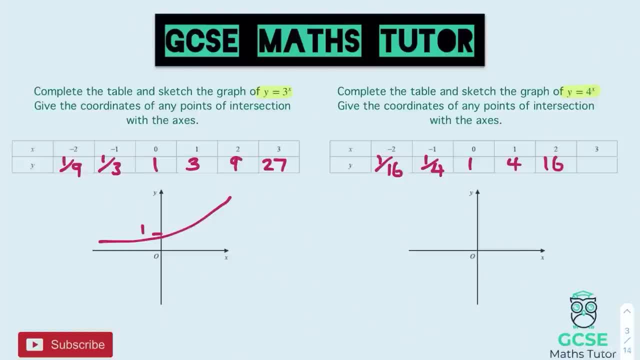 of 3 is 4, well, 16 times 4 again, which is 16.. And again, draw in a sketch and you could emphasise the fact that it's going to be sloping up more. but again, just emphasising it crosses through the y axis at 1.. 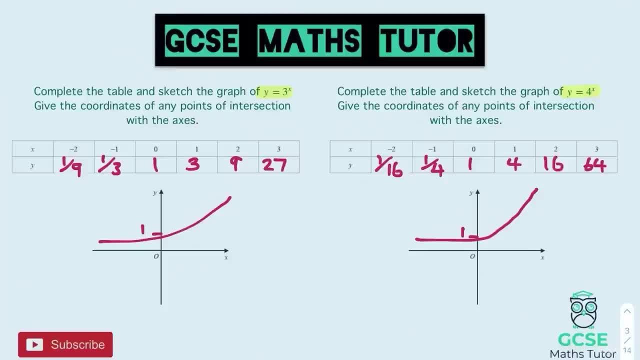 So, as you can see, it's a little bit strange because both my sketches look pretty much the same. but again, we're not drawing it to scale, we're just showing the direction that it's sloping in and also the fact that it crosses the y axis at 1.. 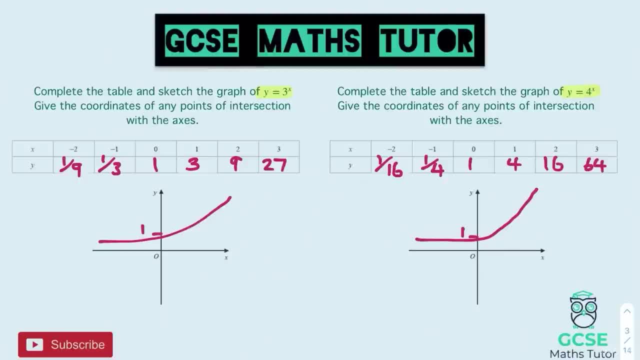 So there we go again. obviously you could have done that ever so slightly differently because you could have put decimals in instead, but obviously that's fine. you should be able to match up your decimals with my fractions there Right Now. let's have a look at a slightly trickier question. 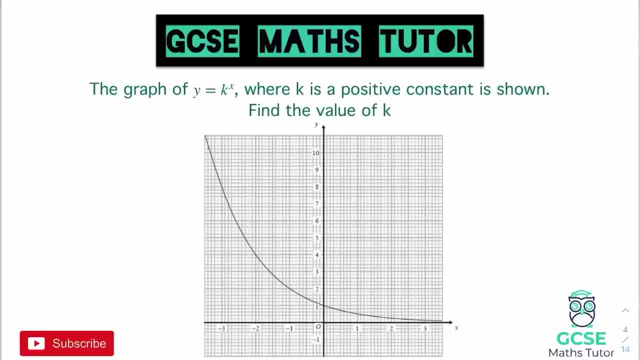 Okay, so here we've got a slightly different question. This is the graph of y. equals k to the power of x, where k as a positive constant is shown. find the value of k. Now that word constant just means that it is not necessarily a whole number. it could. 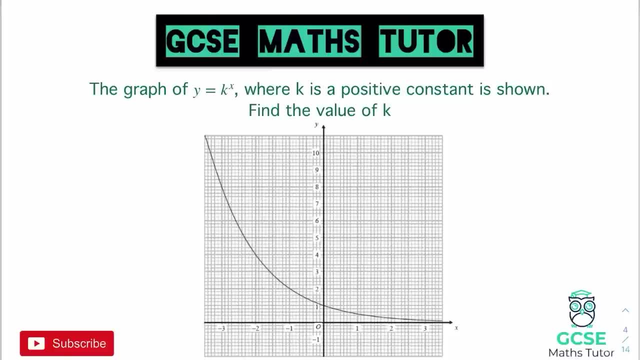 be a fraction as well. So when we're having a look at this, we just need to figure out how we're going to approach it Now, so we know it's going to be. y equals k to the power of something, and we can always. 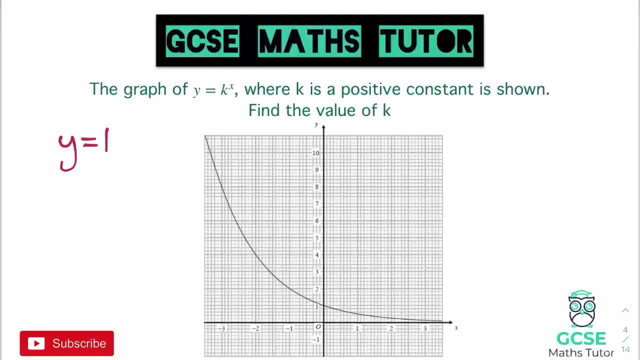 write that down just to remind ourselves of that: y equals k to the power of x. Now, what we're going to do is we're going to try and figure these out, and what we can do is we can pull some coordinates off of our graph. 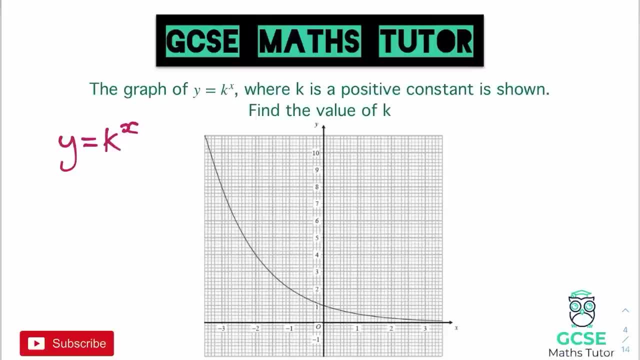 Now we know that, with a graph like this, it's going to go through. This one's slightly different to the ones we were looking at, though, because this one is actually sloping downwards, So something is going to be different in terms of our value of k and that word there, where 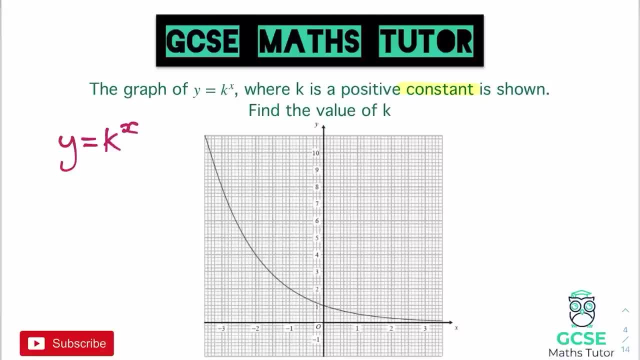 it says constant gives us a little bit of a hint. It means there's not necessarily going to be a whole number, so maybe k is going to be a fraction this time And hopefully, once we've seen this, we'll recognise that these downwards sloping exponential values 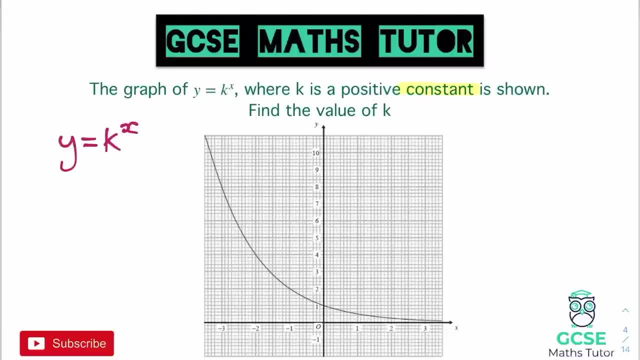 these exponential graphs do have a different value in place of k there. Now, in terms of how we go about this, we could pick the coordinate. let's just have a look at that one and how we'd approach it. Now we know that zero is the x coordinate and y has got a value of one. 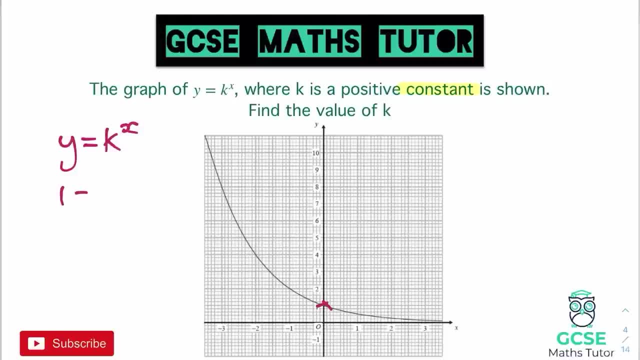 But if we were to plug this into our formula, we would have one, as our y value is equal to k, to the power of zero, And that leaves it a bit open-ended, because we know that no matter what goes in place of that k, we're always going to get the value of one. 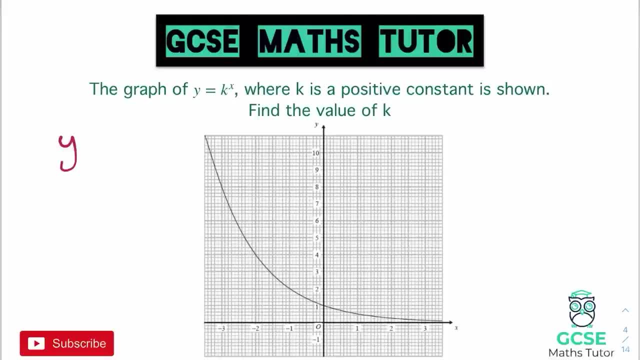 k to the power of something, and we can always write that down just to remind ourselves of that. y equals k to the power of x. Now what we're going to do is we're going to try and figure these out. We can pull some coordinates off of our graph. Now we know that with a graph like this, it's going. 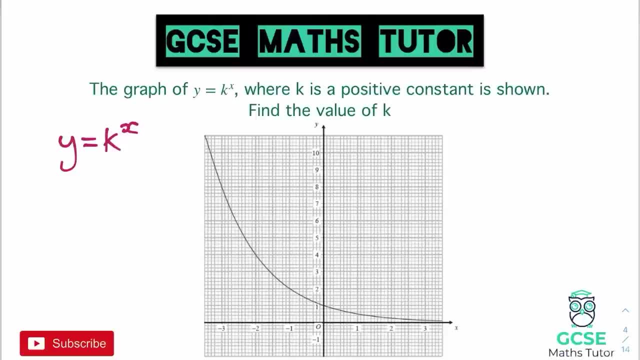 to go through 0,1.. This one's slightly different to the ones we were looking at, though, because this one is actually sloping downwards, So something is going to be different in terms of our value of k, and that word there, where it says constant, gives us a little bit of a hint. 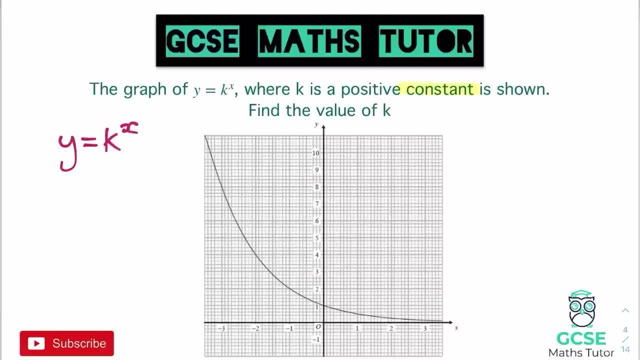 It means there's not necessarily going to be a whole number, so maybe k is going to be a fraction this time, and hopefully, once we've seen this, we'll recognise that these downward sloping exponential graphs do have a different value in place of k there. 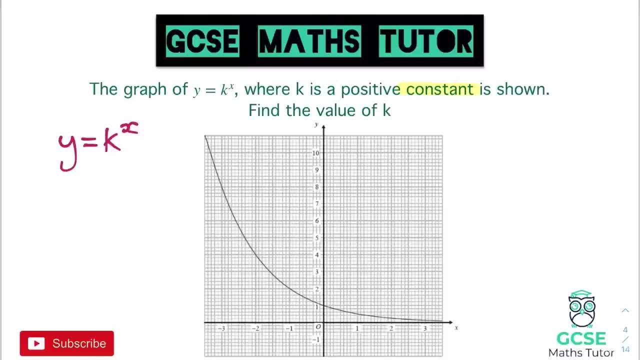 Now, in terms of how we go about this, we could pick the coordinate 0,1.. Let's just have a look at that one, how we'd approach it. Now we know that 0 is the x coordinate and y has got a value of 1. 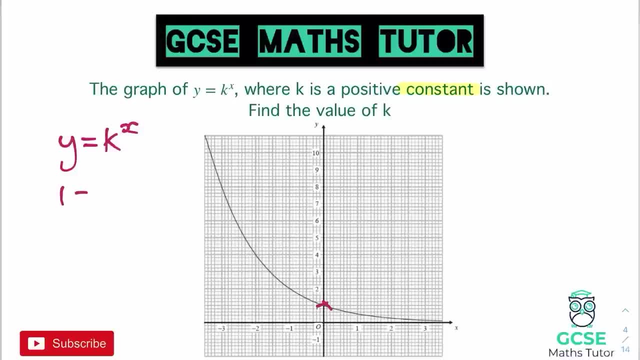 but if we were to plug this into our formula, we would have 1, as our y value is equal to k, to the power of 0, and that leaves it a bit open-ended, because we know that no matter what goes in place of that k, we're always going to get the value of 1.. So that's not particularly 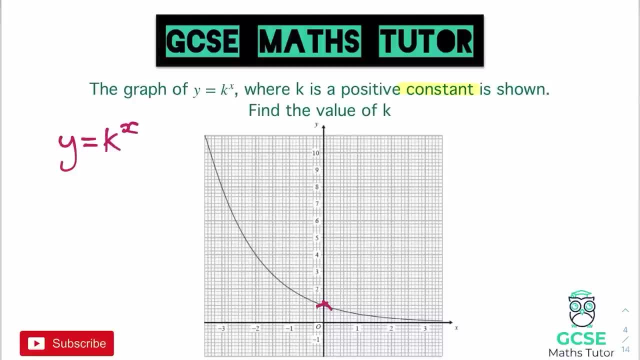 any help to us, so we're going to have to go for a different coordinate. Let's find a different one. Now. there's a couple that I can see here, both in the negative region. I think it's a bit difficult to find a good one in the positive region there, as they're a bit small. 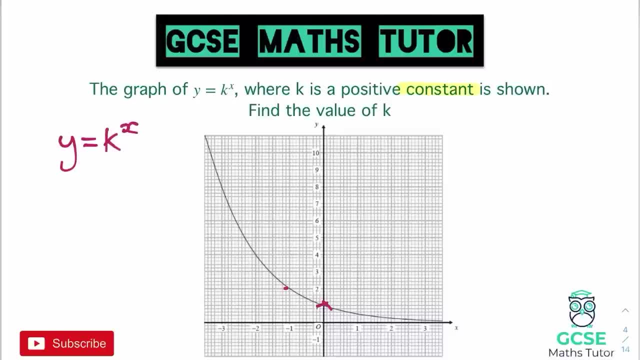 but if we have a look, where does negative 1 land? Negative 1 lands at 2.. So we've got a coordinate there. What about negative 2? That lands at 4.. Maybe negative 3? That lands up here at 8.. 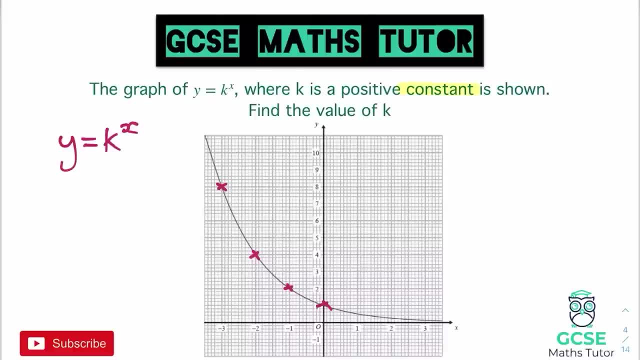 So here we can pick any of those. I'm going to go for the negative 1 being at 2.. So what we have is 2 as our y coordinate. so 2 is equal to k, to the power of our x coordinate there, which is negative 1. and again, here is where. 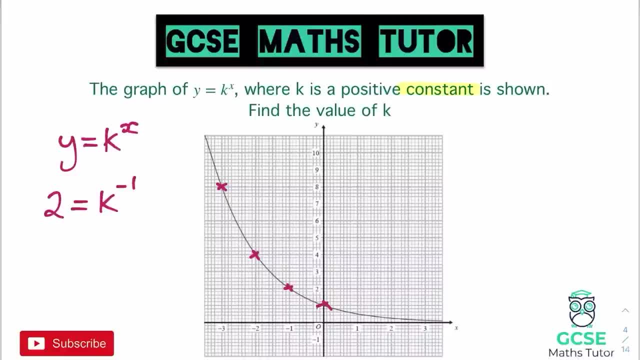 you have to have a really good understanding of your well, I want to say fractional negative indices, but in this case it's just negative indices. So again I'll link that in the description. but this is almost a reverse negative index. So we have to figure out what value to the power. 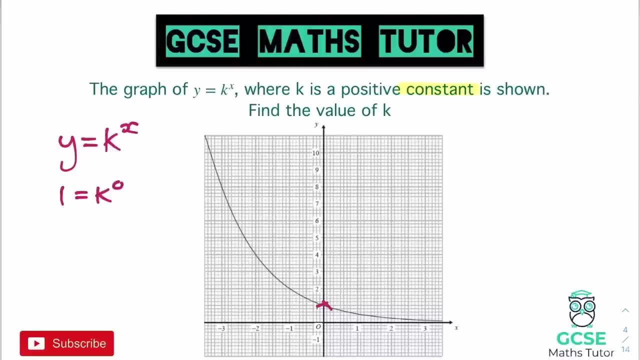 So that's not particularly any help to us. so we're going to have to go for a different coordinate. Let's find a different one. Now. there's a couple that I can see here, both in the negative region. I think it's a bit difficult to find a good one in the positive region there as they're. 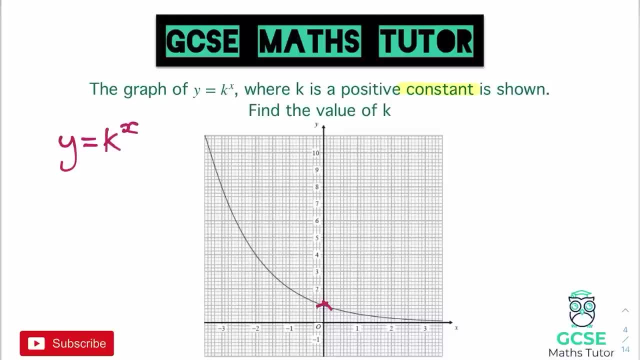 a bit small. But if we have a look, where does negative one land? Negative one lands at two, So we've got a coordinate there. what about negative two That lands at four? Maybe negative three That lands up here at eight? 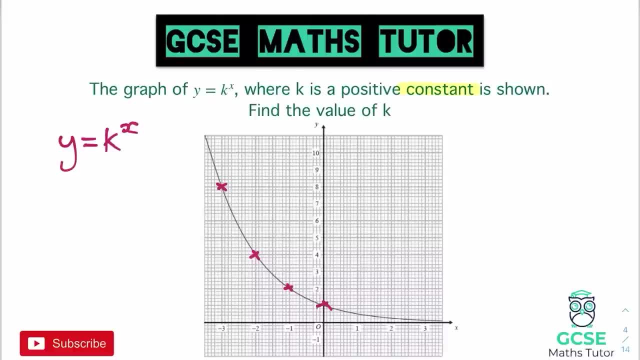 So, anyway, we could pick any of those, I'm going to go for the negative one being at two. So what we have is two is our y coordinate. so two is equal to k, to the power of our x coordinate there, which is negative one. 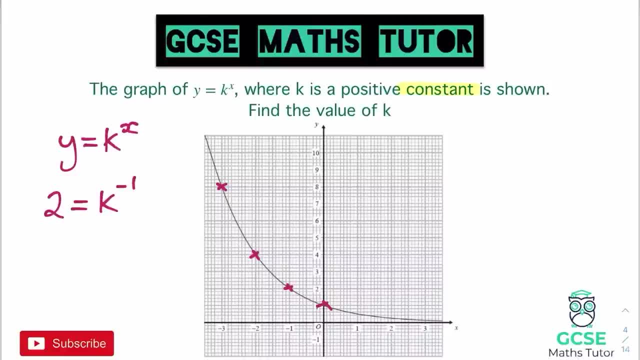 And again, here is where you have to have a really good understanding of your well, I want to say fractional negative indices, but in this case it's just negative indices. So again, I'll link that in the description. but this is almost a reverse negative indices. 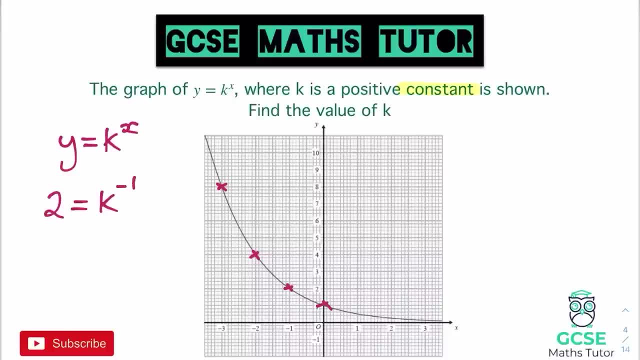 So we have to figure out what value to the power of negative one gives us a value of two And essentially we just have to reverse that power. We know that a negative power does the reciprocal Right Now. at the moment, two is two over one. if we were to write that as a fraction. 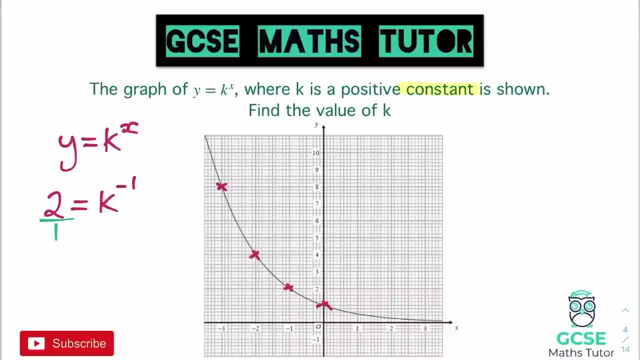 It always looks a bit weird writing it as two over one, but it just helps to visualise that reciprocal. So if we flip that over that becomes a half And obviously it's a power of negative one there. So that means there were no powers involved. 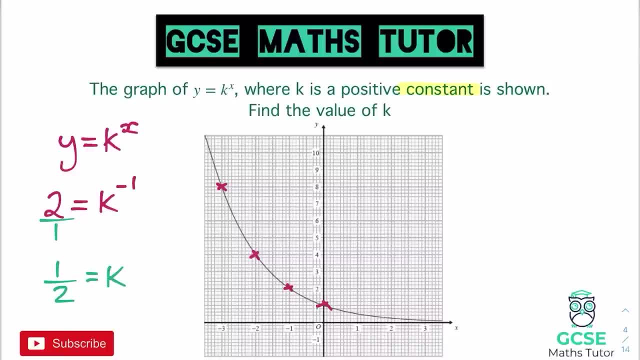 So a half is equal to k or k is equal to a half. Now that's our value there. Let's have a look at maybe, if we depict the negative two, how we'd approach that, because we might not have a nice value on the negative one. 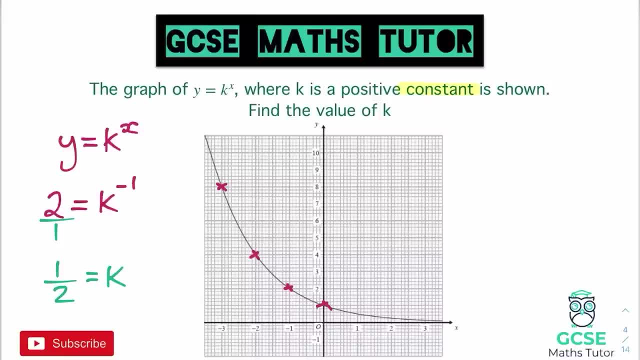 Now, if it was the negative two, we'd have a negative one. So if it was the negative two, which goes up to a value of four, this one here we're looking at now- then I would, instead of putting these values in, so I'd have four is equal. 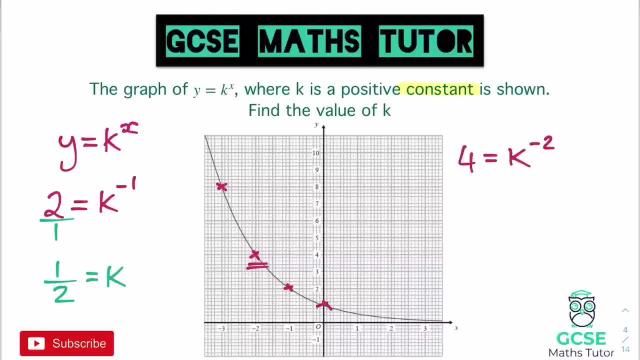 to k to the power of negative two. And again we can take the same approach. We know that four is four over one. there was a reciprocal involved, So if we flip that over we get a quarter which is going to be equal to, not k to the 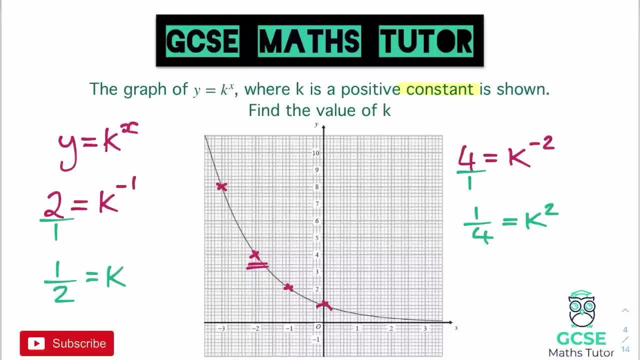 minus two, but just the k squared. Now we've reversed that negative power And in order to get rid of the k squared We would now need to square root both sides. So we'd have to do the square root of both numbers there and we would get one over two. 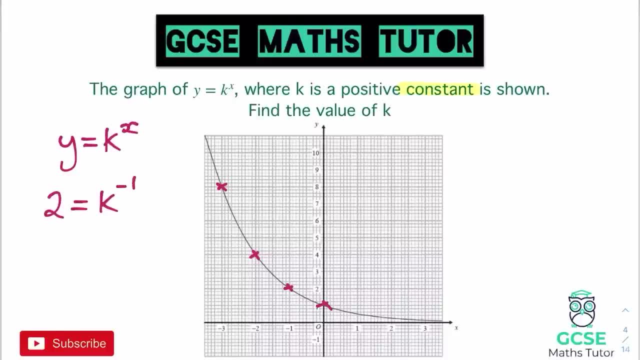 of negative. 1 gives us a value of 2 and essentially we just have to reverse that power. We know that a negative power does the reciprocal. Now, at the moment, 2 is 2 over 1. if we were to write that as a fraction. So if we were to write that as a fraction, it would be 2 over 1.. 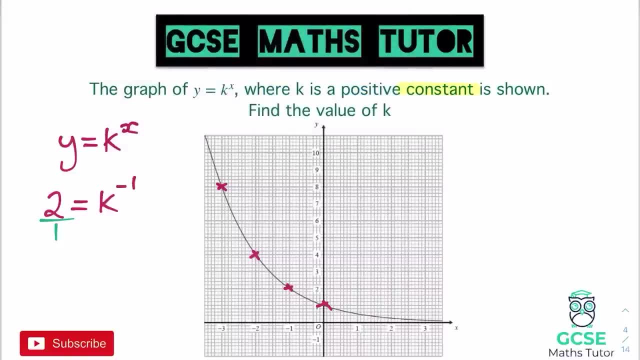 It always looks a bit weird writing it as 2 over 1, but it just helps to visualize that reciprocal. So if we flip that over that becomes a half and obviously it's a power of negative 1 there. so that means there were no powers involved. so a half is equal to k or k is equal to a half. 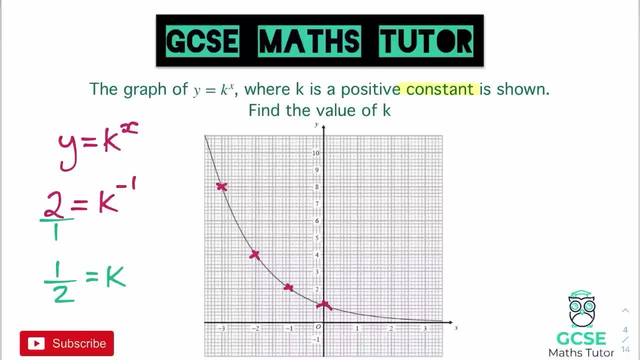 Now that's our value there. Let's have a look at maybe, if we depict the negative 2, how we'd approach that, because we might not have a nice value on the negative 1.. Now, if it was the negative 2, which goes up to a value of 4- this one here we're looking at now, 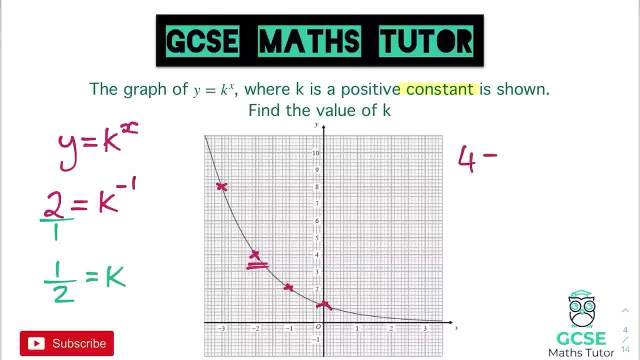 then I would, instead of putting these values in, so I would have: 4 is equal to k, to the power of negative 2, and again we can take the same approach. We know that 4 is 4 over 1, there was a reciprocal involved. so if we flip that over, we get a quarter. 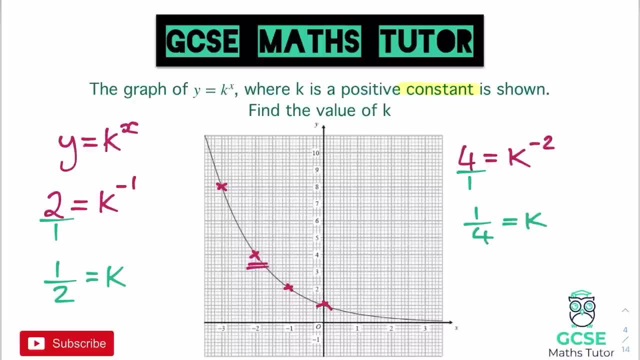 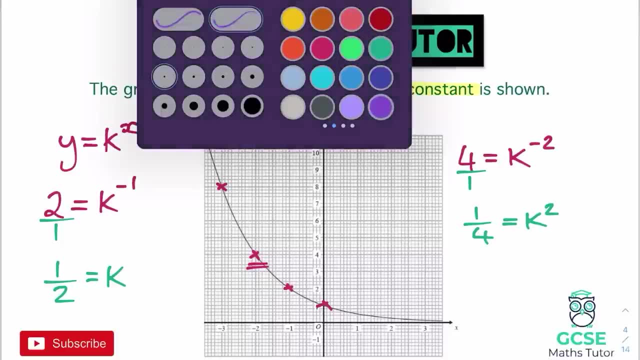 which is going to be equal to not k to the minus 2, but just the k squared. Now we've reversed that negative power and in order to get rid of the k squared we would now need to square root both sides, So we would have to do the square root of both numbers there. 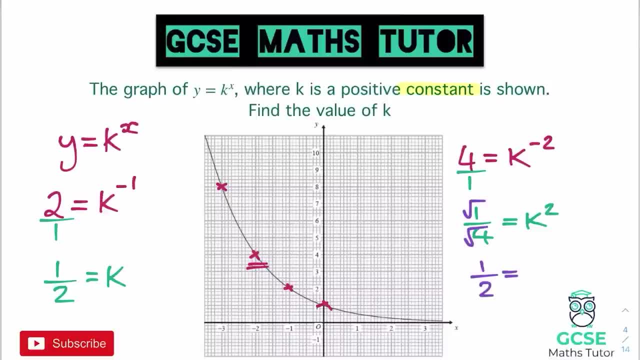 there and we would get 1 over 2, which is equal to k. And there we go. we've found that value of k- k is equal to a half. So this is really just highlighting a different technique that we might have to use with some of these harder questions where we might just have to pull. 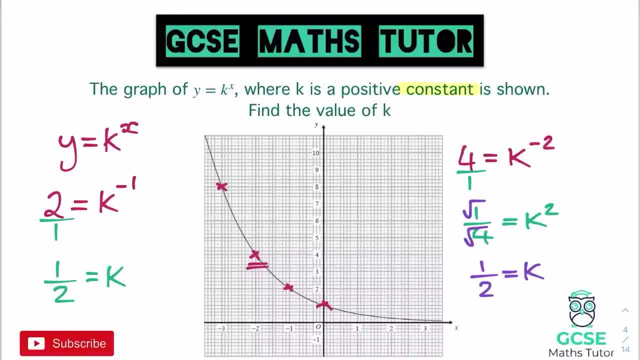 a coordinate off the graph and sub it into that equation. So these ones are okay actually to approach, but we're going to have a look at something slightly trickier to this to finish off for our final question. So let's have a look at that now. Okay, so this question. 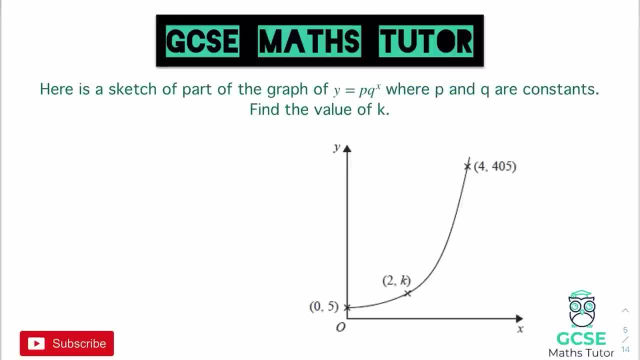 here gives us two very specific coordinates on our graph, or three if we consider the one on the y intercept, which is going to be crucial for this question, And you're going to have a practice at one of these questions in a sec, so do make sure you are making some notes. 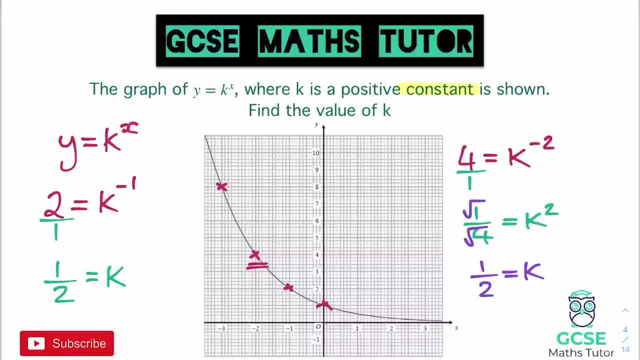 which is equal to k. And there we go. we found that value of k, k is equal to a half. So this is really just highlighting a different technique that we might have to use with some of these harder questions where we might just have to pull a coordinate off the graph. 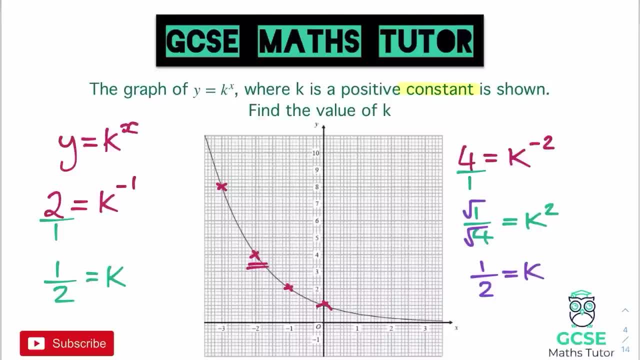 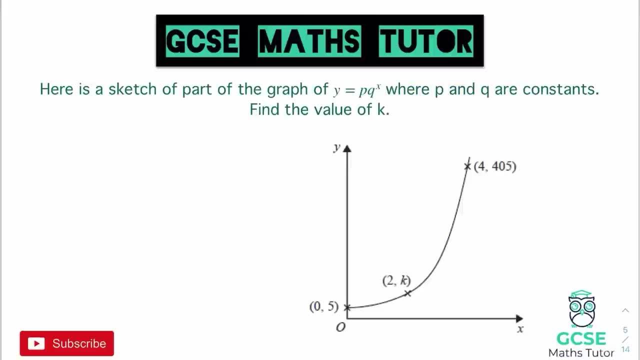 and sub it into that equation. So these ones are okay actually to approach, but we're going to have a look at something slightly trickier to this. to finish off for our final question, Let's have a look at that now. Okay, so this question here gives us two very specific coordinates on our graph, or three. 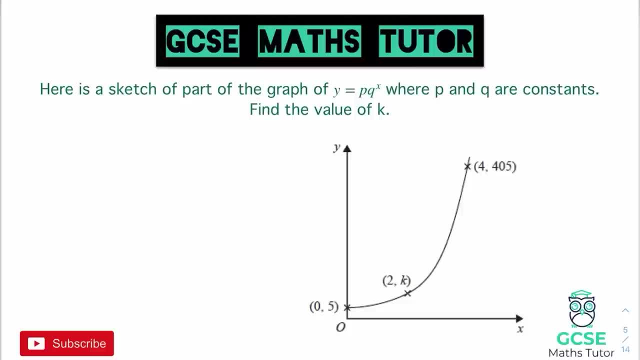 if we consider the one on the y intercept, which is going to be crucial for this question- And you're going to have a practice at one of these questions in a sec, so do make sure you are making some notes on this one. It says- here is a sketch of part of the graph of: y equals pq to the power of x, where p. 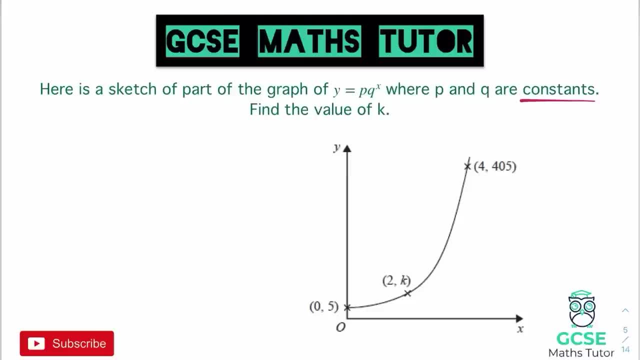 and q are constants. Again, it uses this word constants here, And this time we have a slightly different equation where we've got y equals pq to the power of x, rather than just maybe q to the power of x, And it says: find the value of k. 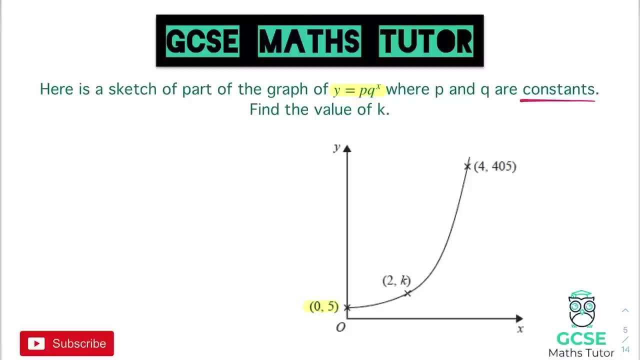 Now this is where this coordinate here on the y axis is going to be really important, because obviously you'll notice that this one changes the rules for us. It doesn't go through, but instead it goes through. Now that means, and if we think about this logically- and here's our equation- y equals. 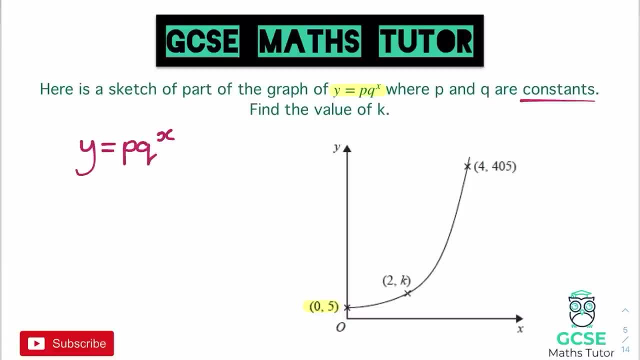 pq to the power of x. Now, whatever q is, as long as we put that power of zero in there, y would have to equal the value of 1.. So, in other words, q to the power of x, when we put zero in, has to equal 1.. 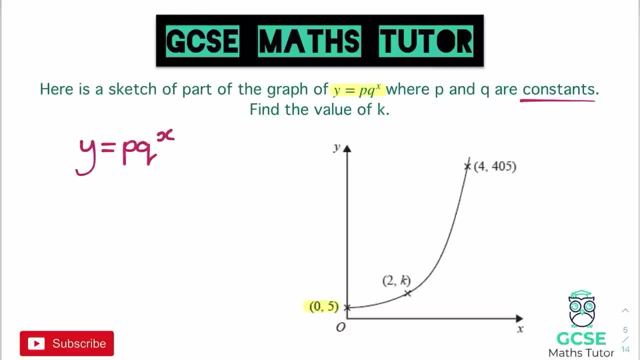 Now that means that in order to change that into a 5, we would have to multiply this q to the power of x part by 5.. And therefore p must be 5.. OK, Let's just break that down. We've got p times q to the power of zero has to equal that y coordinate, which is 5.. 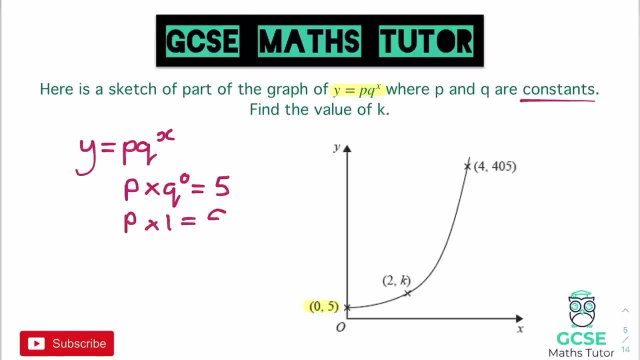 Or p times 1 equals 5.. So therefore, p has to equal 5.. So that's the equation. So therefore p has to equal 5.. Now you don't really have to write the working out down there. If you see the logic in that, you can see that p has to equal 5 in order to shift that. 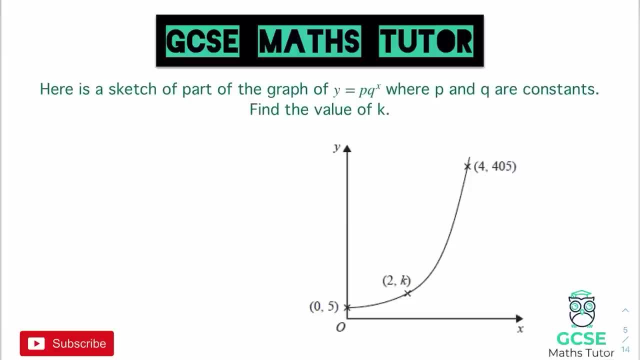 on this one. It says: here is a sketch of part of the graph of: y equals pq to the power of x, where p and q are constants. Again, it uses this word constants here, And this time we have a slightly different equation. We've got y equals pq to the power of x rather than 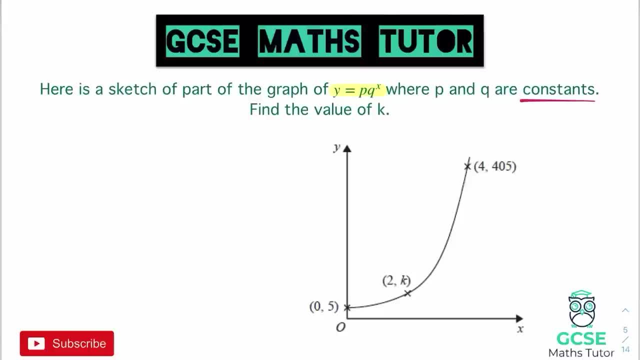 just maybe q to the power of x, and it says: find the value of k. Now this is where this coordinate here on the y axis is going to be really important, because obviously you'll notice that this one changes the rules for us. It doesn't go. 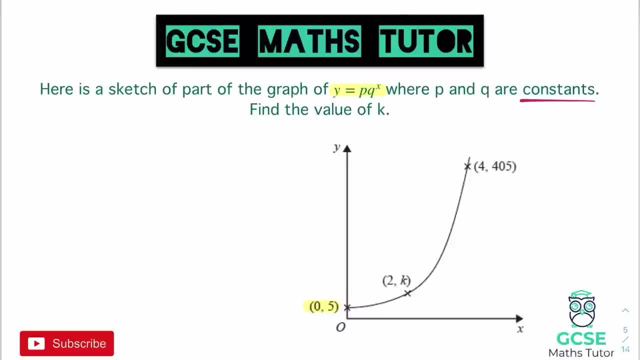 through, but instead it goes through. Now that means, and if we think about this logically- and here's our equation- y equals pq to the power of x. Now, whatever q is, as long as we put that power of 0 in there, y would have to equal a value of 1.. Or in other, 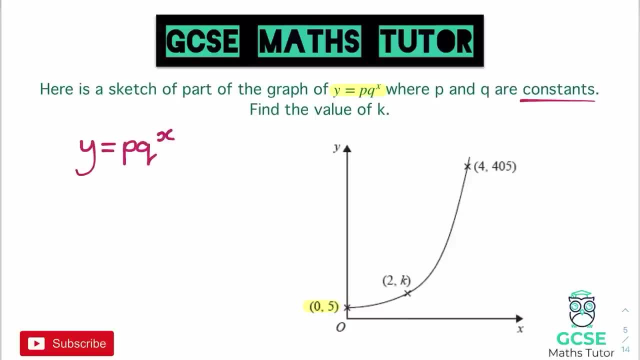 words q to the power of x. When we put 0 in it has to equal 1.. Now that means that in order to change that into a 5, we would have to multiply this q to the power of x part by 5.. And therefore p must. 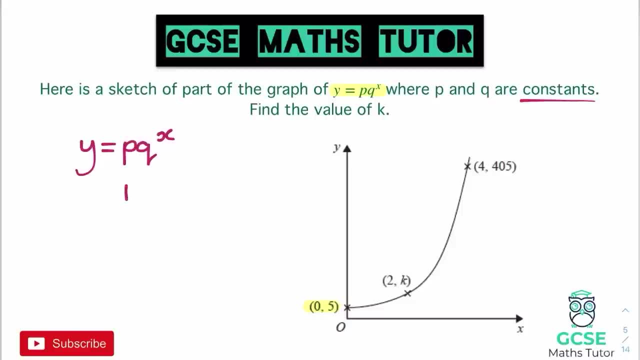 be 5.. Let's just break that down. We've got p times q to the power of 0 has to equal that y coordinate, which is 5.. Or p times 1 equals 5. so therefore p has to equal 5.. Now you don't really have. 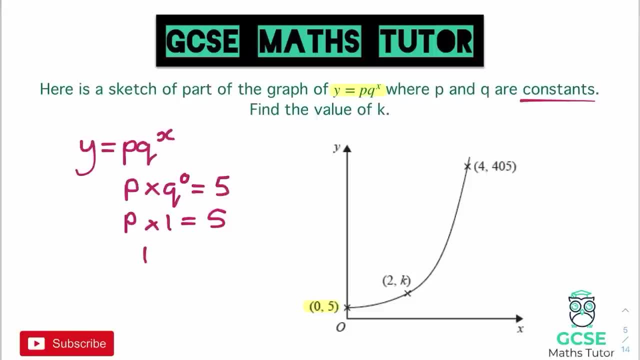 to write the working out down there. if you see the logic in that, you can see that p has to equal 5 in order to shift that y intercept up to that value of 5.. So let's get rid of this working. Just a little bit of logic there, so we'll have a look at this now. So we've got p equals. 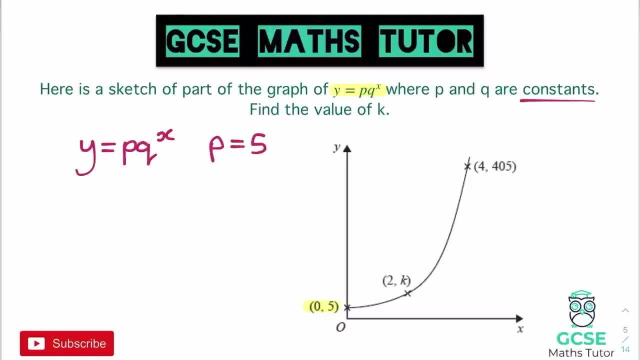 5.. Now, if we rewrite this equation, then we now have y equals p, which is 5, and then q to the power of x or 5 times q to the power of x. Now we can go about actually trying to figure this out. 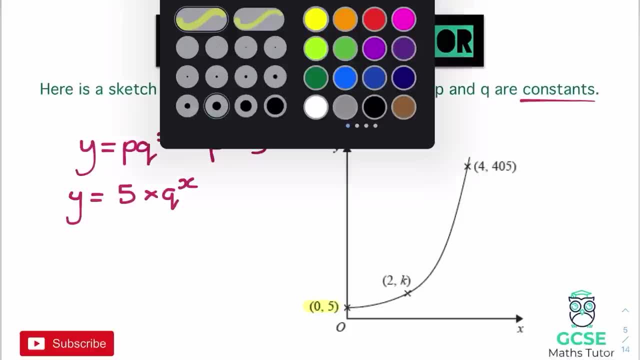 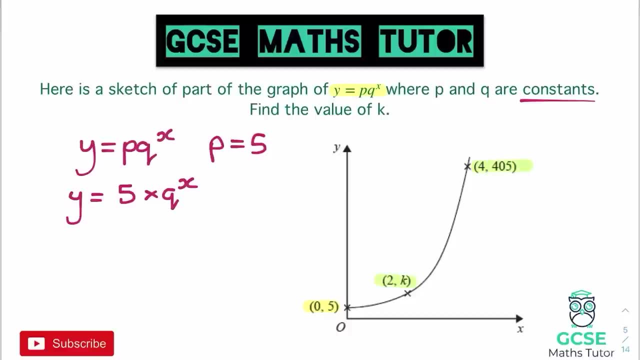 So we've been given some coordinates. Now we've been given two more. Let's highlight this in a different colour. We've got 2 and k, and we've got 4 and 405.. Now obviously we're trying to work out the value of k. so substituting that coordinate into our equation isn't necessarily. 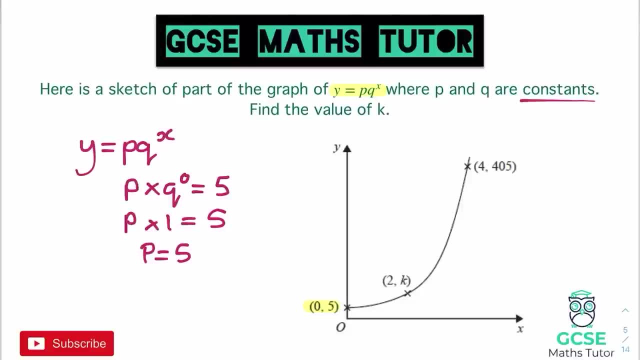 y intercept up to that value of 5.. So let's get rid of this working. Just a little bit of logic there, So we'll have a look at this now. So we've got p equals 5.. Now if we rewrite this equation, then we now have y equals p, which is 5, and then q to 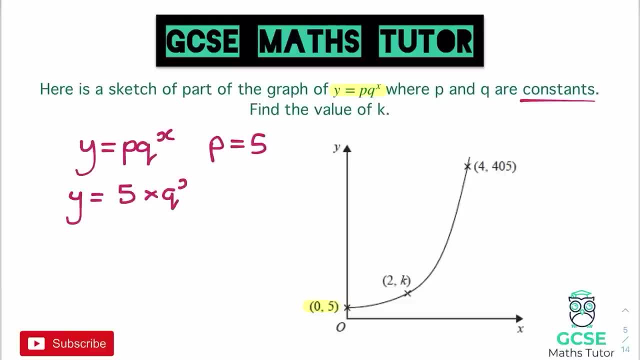 the power of x, or 5 times q to the power of x. Now we can go about actually trying to figure this out, because we've been given some coordinates, Now we've been given two more. Let's highlight this in a different colour. 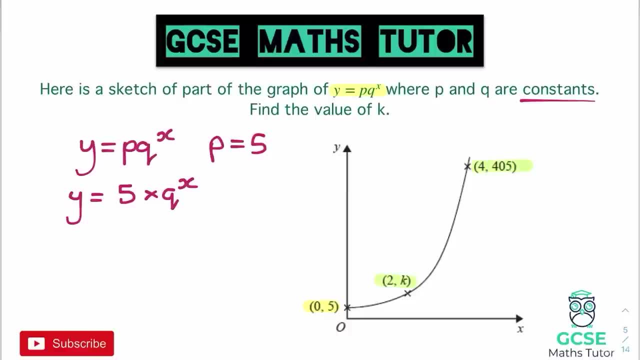 We've got 2 and k and we've got 4 and 405.. Now obviously we're trying to work out the value of k, so substituting that coordinate into our equation isn't necessarily going to help us find what we're looking for. which. 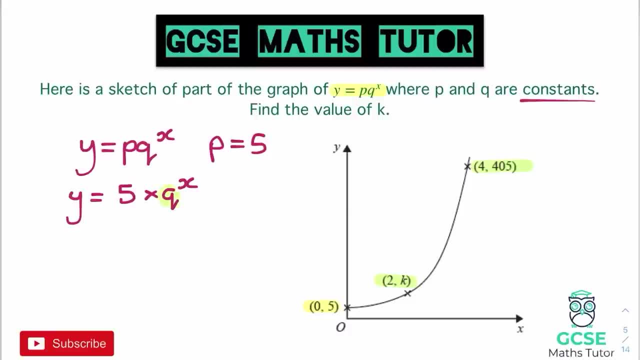 in this case is this value of q, so that we can then go ahead and obviously find that value of k. So if we have a look here, let's plug this coordinate in. So 4 is our x coordinate and 405 is our y coordinate. 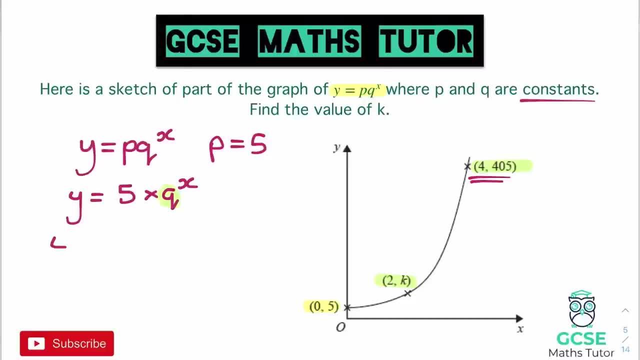 So if y is our x coordinate, then 405 is our y coordinate. So if y is our x coordinate, then 405 is our y coordinate. So if y is our x coordinate, then 405 is our y coordinate. So if y is 405, we have 405 equals 5 times q to the power of the x coordinate, which. 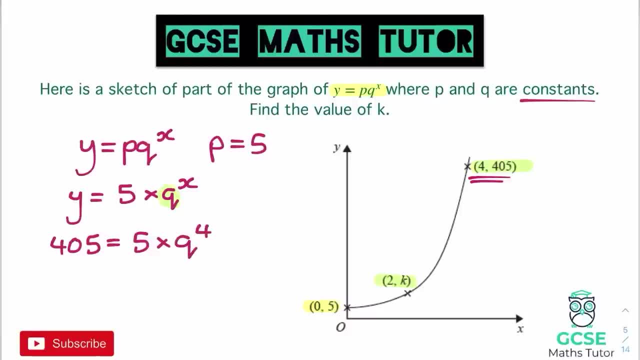 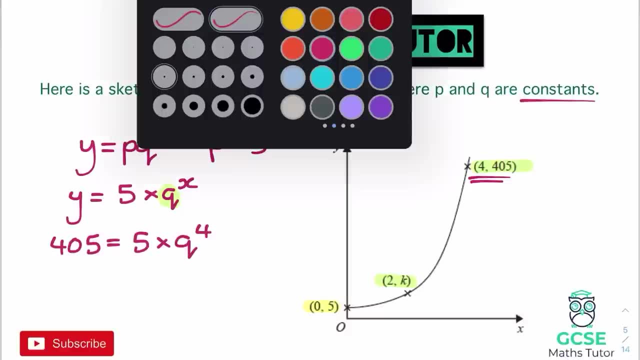 is 4.. And now we just need to unravel this or reverse the process. So, as we are multiplying by 5 on the right hand side there, we can divide both sides by 5.. Let's just write this step of working out down: we'll divide by 5.. 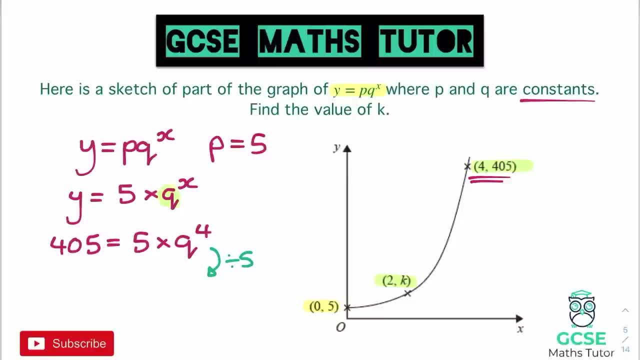 If we divide by 5, we can do 405 divided by 5, which is 81, and we get: 81 is equal to q, to the power of 4.. There we go, we've got something: to the power of 4 equals 81. 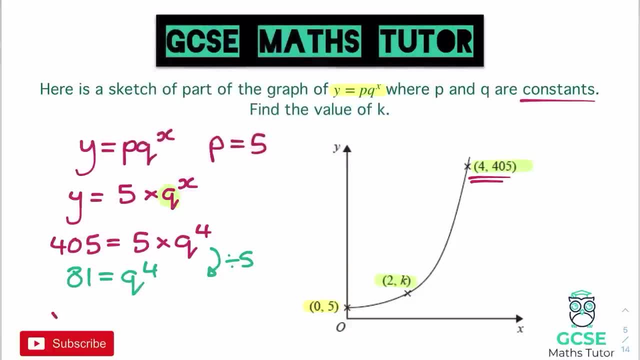 Now you might know what that is. If you don't, then we're going to have to do a fourth root. So we'll do the fourth root of 81, which is equal to 3.. So there we go. q has to equal 3.. 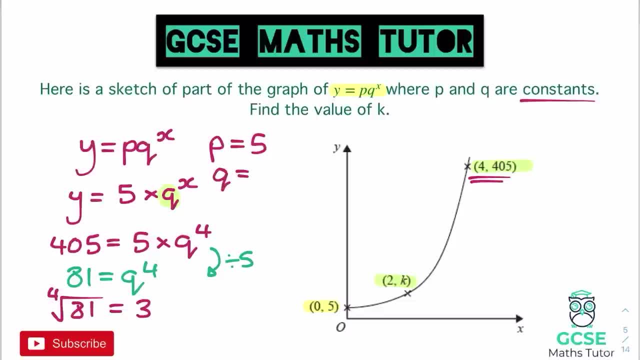 And we can write that at the top here. we've got now q equals 3.. So we've got our two values, so we can actually now write out the full equation. So instead of having all of this working out, we've now got that y is equal to 3.. 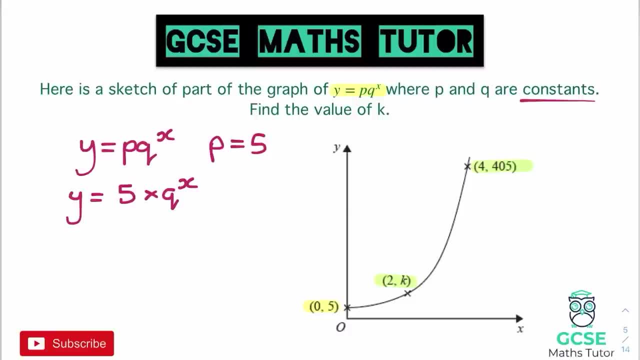 going to help us find what we're looking for, which, in this case, is this value of q, so that we can then go ahead and obviously find that value of k. So if we have a look here, let's plug this coordinate in. So 4 is our x coordinate and 405 is our y coordinate. So if y is 405, 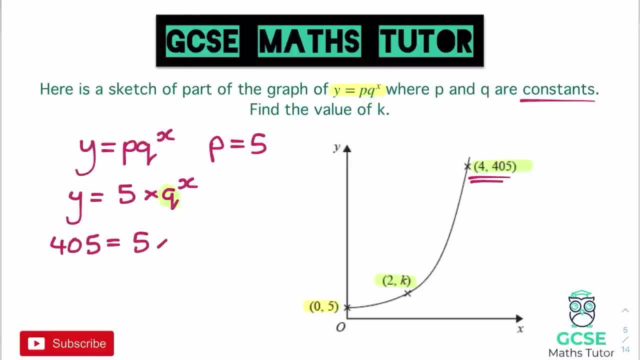 we have 405.. So we've got: p equals 5 times q to the power of the x coordinate, which is 4.. And now we just need to unravel this or reverse the process, So as we are multiplying by 5 on the right, 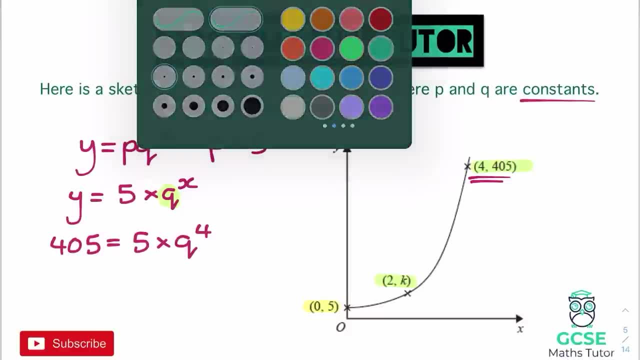 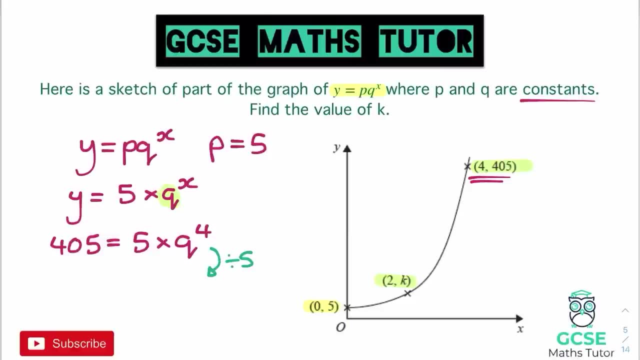 hand side. there we can divide both sides by 5.. Let's just write this step of working out down. We'll divide by 5.. If we divide by 5, we can do 405 divided by 5, which is 81, and we get. 81 is equal to q. 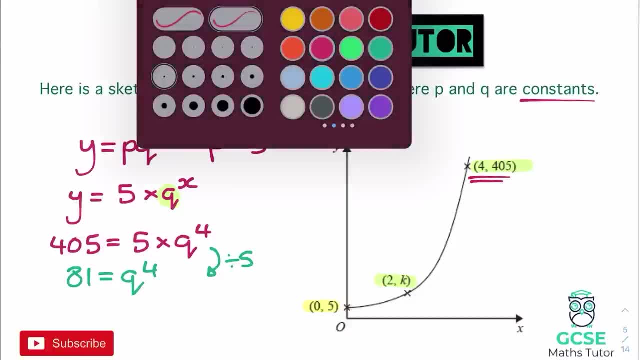 to the power of 4.. There we go, We've got something to the power of 4 equals 81. Now you might know what that is. if you don't, then we're going to have to do a fourth root, so we'll do the fourth. 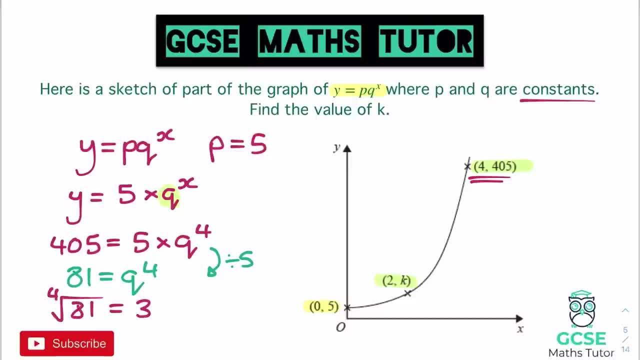 root of 81, which is equal to three. So there we go. q has to equal 3.. And we can write that at the top here. we've now got q equals 3.. So we've got our two values, so we can actually write out the full equation. So instead of having all of this working out, we've now got that y is equal to p, which is 5 minus 4.. And then now we're going to write the x coordinate. So if this is equal to c, it's now equal to 10.. And now we've actually got, if we're going. 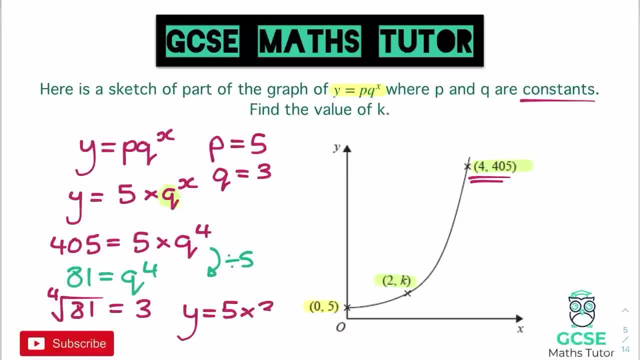 to be writing this around. the new equation. we've now got q as capital and plus 1 hat equal, multiplied by 3, to the power of x, and that makes it nice and simple now for us to work out our final value here that we're looking for. So if we look at our final coordinate, we've got 2 and k. 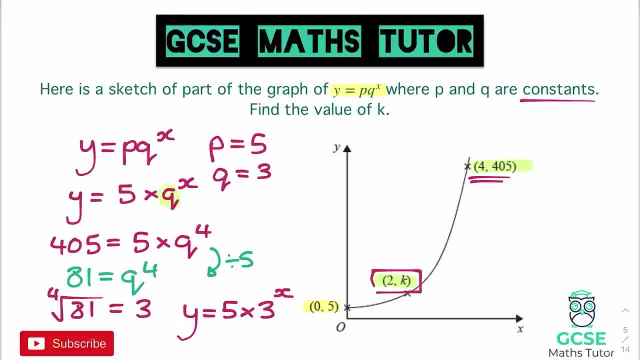 so 2 is our x coordinate and k is our y coordinate. so plugging that into this equation here, our y equals 5 to the power, 5 times 3 to the power of x. instead we'll have: k is equal to 5 times 3 to. 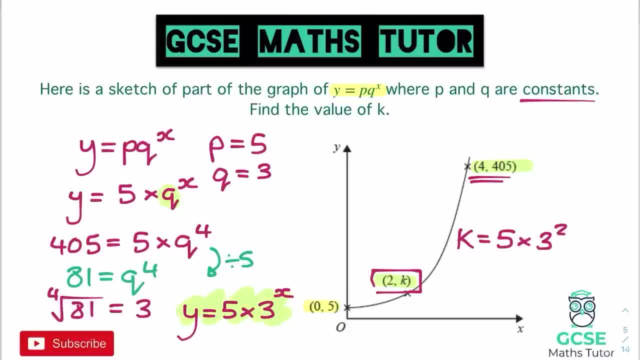 the power of 2 or 3 squared. and if we work that out, 5 times 3 squared, 3 squared is 9. 5 times 9 is 45, so k is equal to 45 and there's our final answer. Okay, so a very similar process to what we. 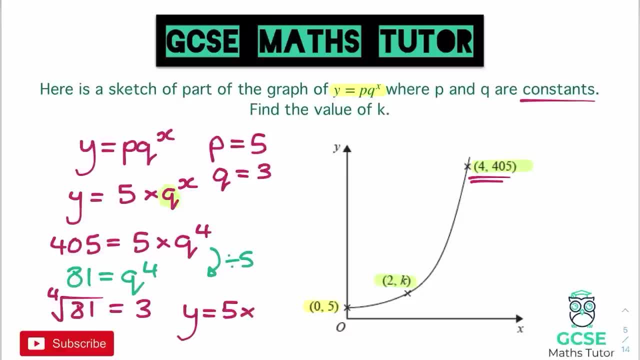 Up to 3 is equal to p, which is 5, multiplied by 3 to the power of x. That makes it nice and simple. now for us to work out our final value here that we're looking for. So if we look at our final coordinate, we've got 2 and k. 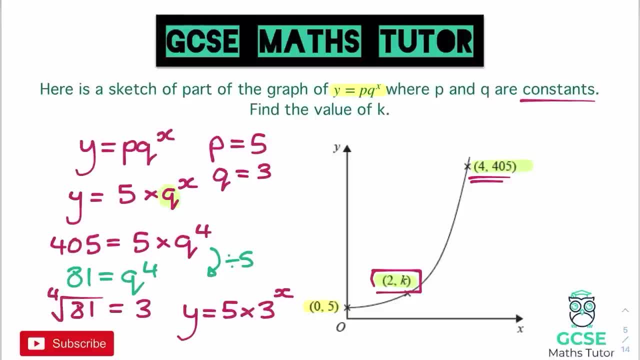 So 2 is our x coordinate and k is our y coordinate. So plugging that into this equation here, our y equals 5 times 3 to the power of x. instead we'll have: k is equal to 5 times 3 to the power of x. 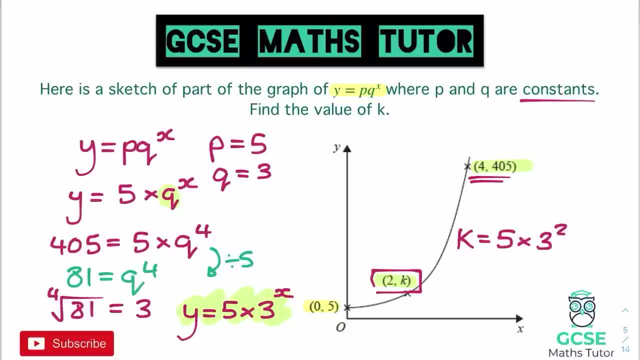 So that means we have the right answer here. So we've got our 4. of 2, or 3 squared, And if we work that out 5 times 3 squared, 3 squared is 9, 5 times. 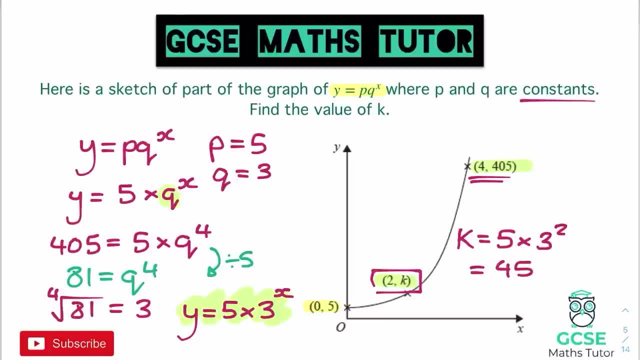 9 is 45. So k is equal to 45, and there's our final answer. So a very similar process to what we used in the previous question, obviously subbing coordinates into our equation there to find out some missing values. But this one was a little trickier here because 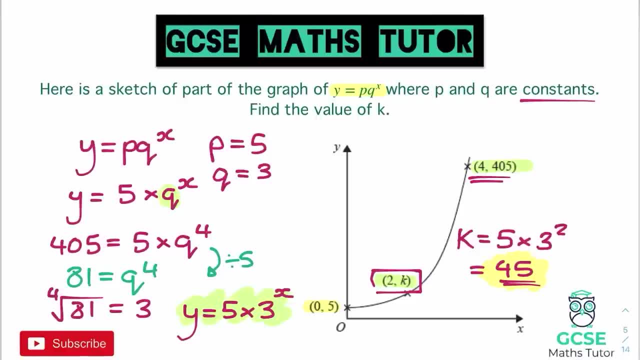 we first had to use a bit of logic to find that value of p, Obviously looking at the y intercept there, it had to multiply it by 5 in order to move it up there, And then obviously we subbed in one coordinate to find out our other missing value and then used: 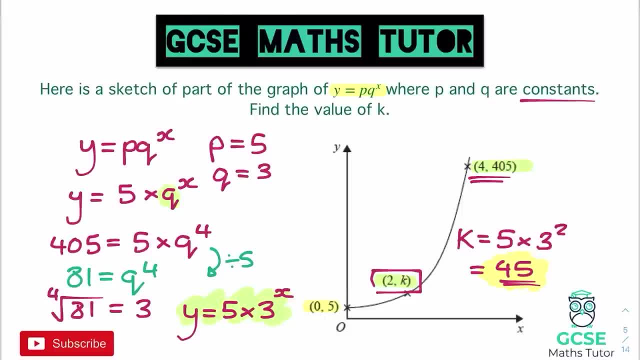 that equation, to find this missing coordinate here, which was k in this question. So there we go. hopefully you made some good notes on that. hopefully that was okay. These are quite tricky questions, but I've got one question for you to have a go at to finish off this. 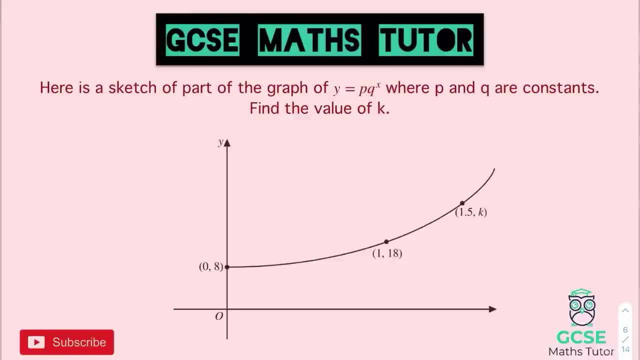 little video on exponential graphs. Okay, so this question here is very similar to the one that we just looked at. We've just got some different coordinates on our curve and just a little bit of logic here. So we've got a little bit of logic here and we've got some different coordinates on our curve and just a little bit of logic here. So we've just got some different coordinates on our curve and we've got some different coordinates on our curve and we've got some different coordinates on our curve. So we've just 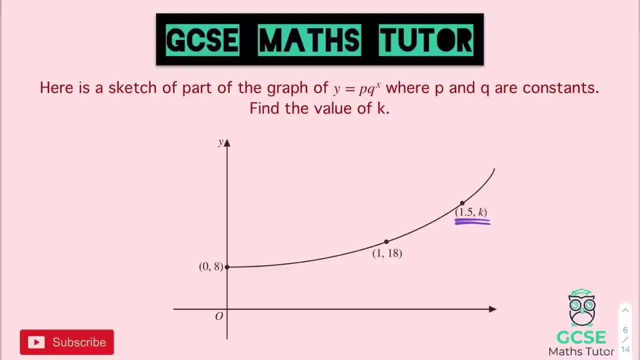 taken note of the fact that the one over here we have got a bit of a decimal, but don't worry about that, it's just a number and you are using a calculator. So pause the video there. have a go at this question and we will go over the answer in a sec. Okay, 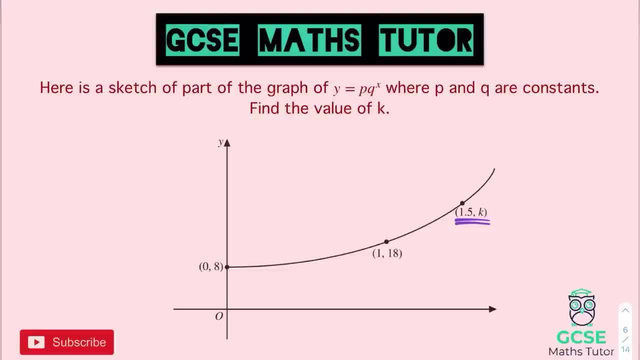 so let's go over the answer for this then. So first thing to note is that it goes up to 8 on the y intercept, and that means this time, rather than having that p value being 5,, our p value is going to be 8, because q to the power of 0 is 1, and our y coordinate. 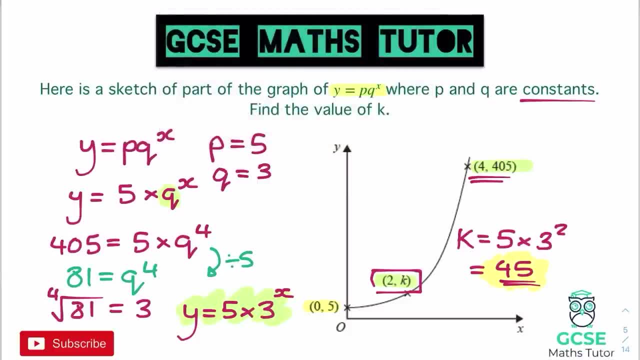 used in the previous question, obviously subbing coordinates into our equation there to find out some missing values. but this one was a little trickier here because we first had to use a bit of logic to find that value of p. obviously, looking at the y intercept there, it had to. 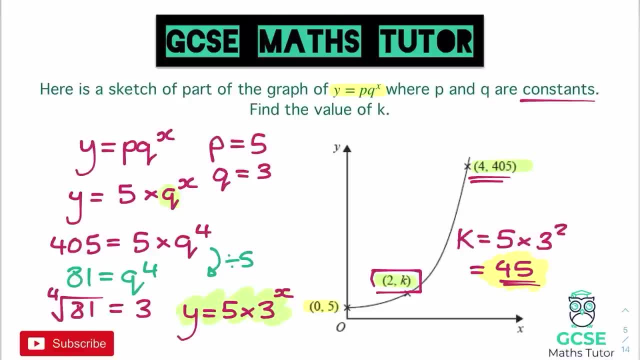 look like this. So if we look at the y intercept there, it had to look like this. So if we look at the y intercept there, it had to look like this. So if we look at the y intercept there, it had to look like: multiply it by 5 in order to move it up there, and then obviously we subbed in one coordinate to: 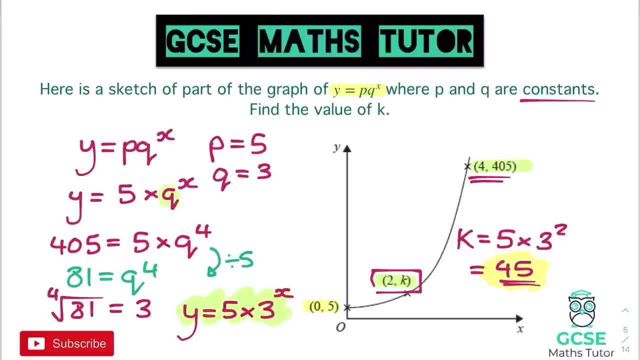 find out our other missing value and then use that equation to find this missing coordinate here, which was k in this question. So there we go. hopefully you made some good notes on that. hopefully that was okay. these are quite tricky questions, but I've got one question for you to. 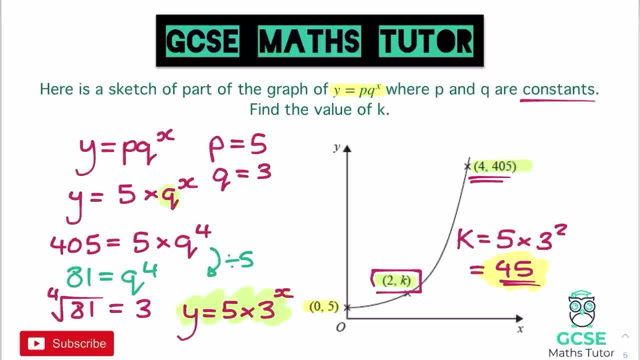 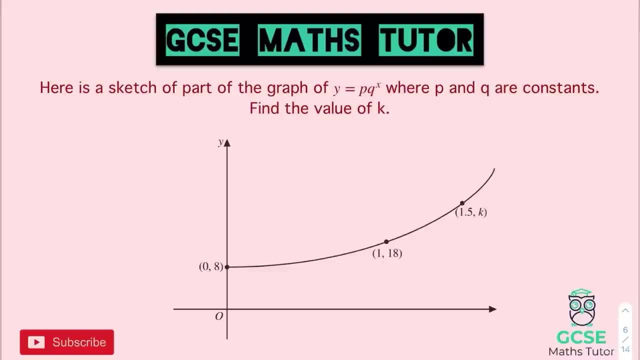 have a go at, to finish off, this little video on exponential graphs. Okay, so this question here is very similar to the one that we just looked at. we've just got some different coordinates on our over here. we have got a bit of a decimal, but don't worry about that, it's just a number and you are. 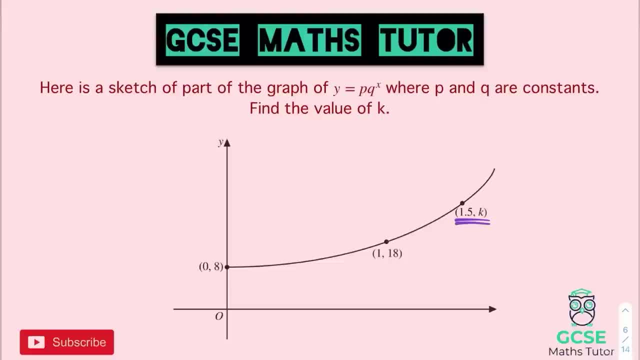 using a calculator, So pause the video there. have a go at this question and we will go over the answer in a sec. Okay, so let's go over the answer for this then. So first thing to note is that it goes up to 8 on the y intercept, and that means this time, rather than having that p value being 5, our 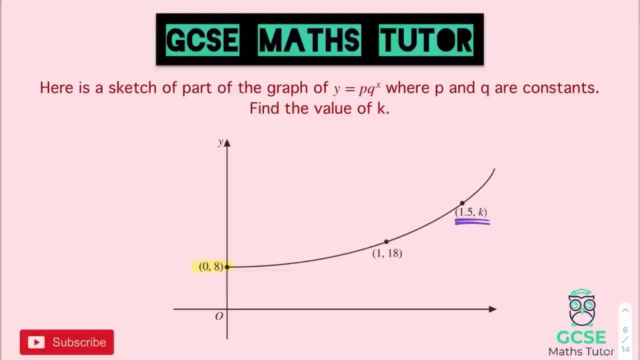 p value is going to be 8 because q to the power of 0 is 1 and our y coordinate has to equal 8. so 8 times 1 p will have to be 8.. So let's write that down: p equals 8.. Writing our equation. then, with our value of p, we've got y. 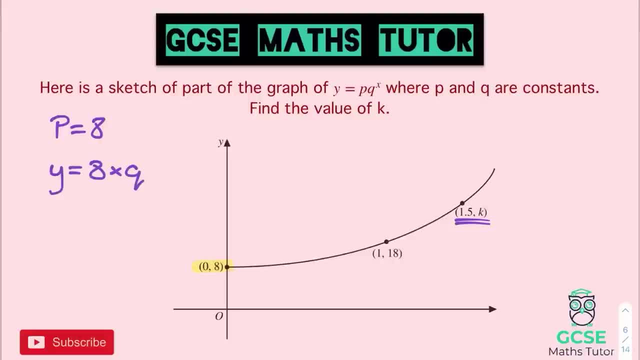 equals 8 times q to the power of x or 8qx. Now what coordinate can we substitute in? because we have 1 and 18 this time on the lower part of the graph. so that's fine, we can sub that in. so we've. 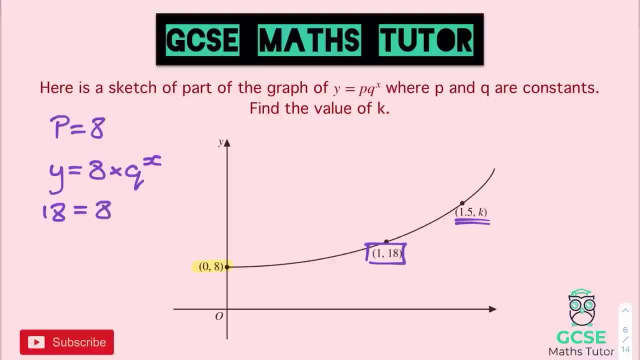 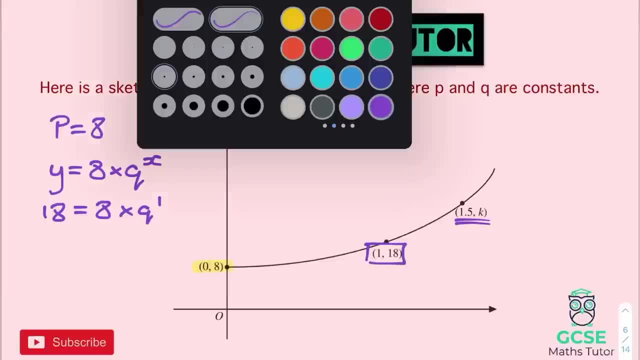 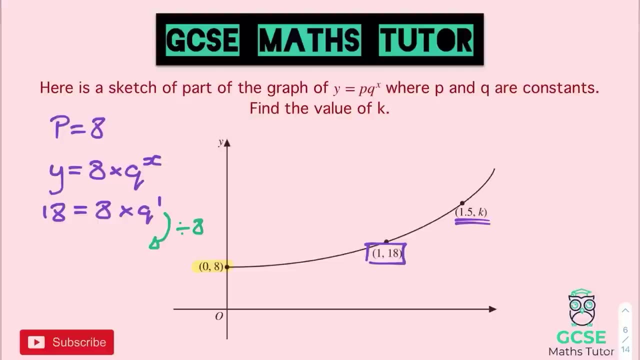 got. 18 equals 8 times q to the power of 1.. We're multiplying by 8 this time, so in order to get that down to just being q on that side, we're going to have to divide both sides by 8.. So 18 divided by 8. again, you can do that on the calculator. 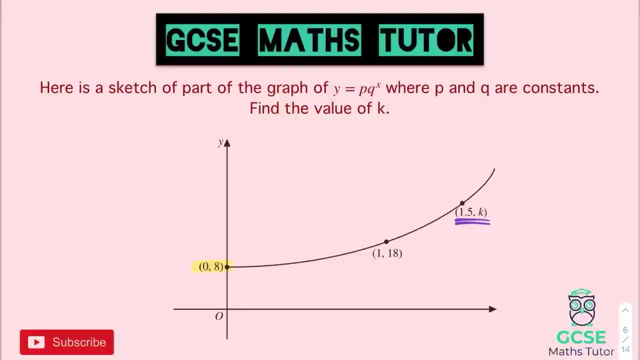 has to equal 8,. so 8 times 1 is going to be 1, and that means that our y coordinate has 1, p will have to be 8.. So let's write that down: p equals 8.. Writing our equation then: 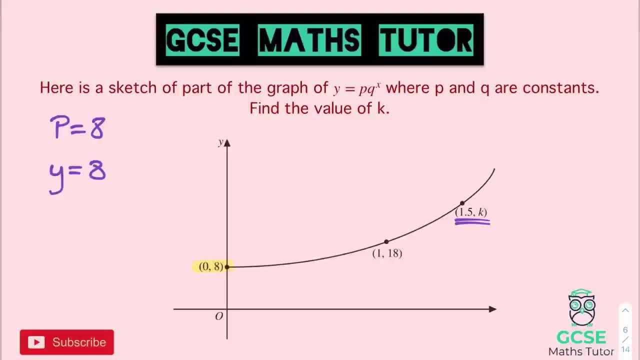 with our value of p, we've got y equals 8 times q to the power of x or 8qx. Now what coordinate can we substitute in? Because we have 1 and 18, this time on the lower part of the graph, so that's fine, we can sub that in. So we've got 18 equals 8 times q. 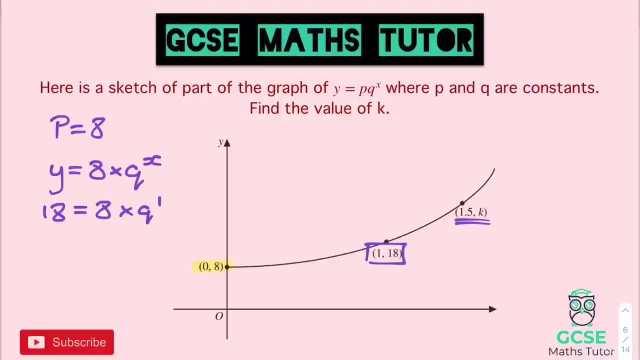 to the power of 1.. Okay, that's fine. We're multiplying by 8 this time. so in order to get that down to just being q on that side, we're going to have to divide both sides by 8.. So 18 divided by 8, again, you can do that on the calculator or you could write it as: 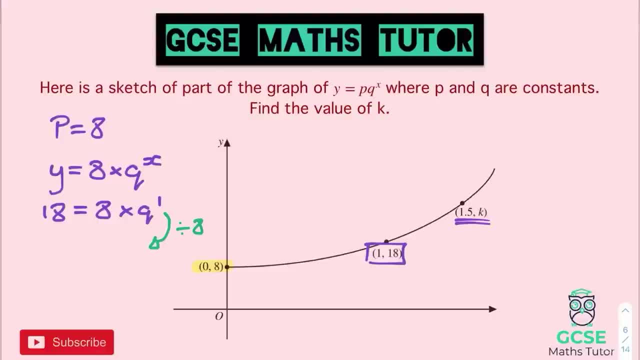 a fraction as well, but this is a calculator question, so we'll stick with using a calculator. So divide 18 by 8, you get 2.25.. So we have: 2.25 is equal to q to the power of 1, so we'll. 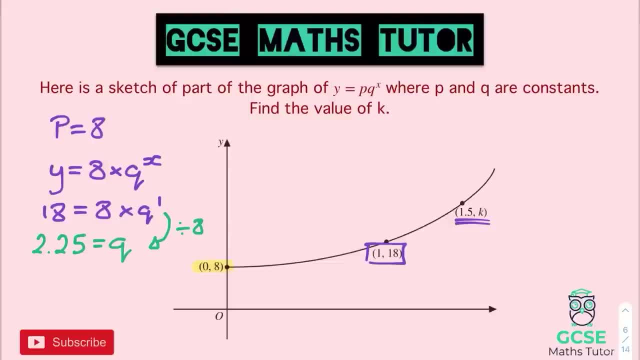 just leave that as q. So there we go. we've got our p value And our q value and now we can write our equation. So let's write our equation down. We've got: y is equal to p, which is 8, multiplied by q, which is 2.25 to the power of x, And 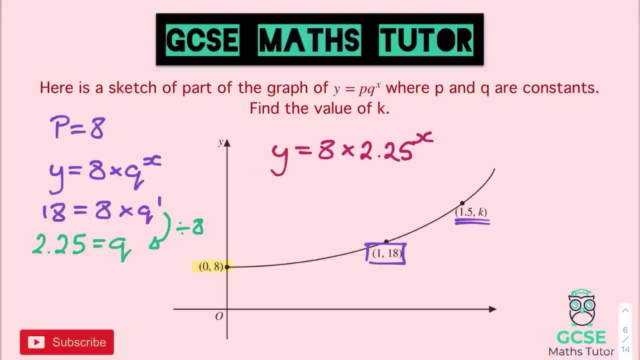 again we're trying to find that value of k, and in this question x is 1.5, and again y is our value of k. So if we substitute those in we get k equals 8 times 2.25 to the power. 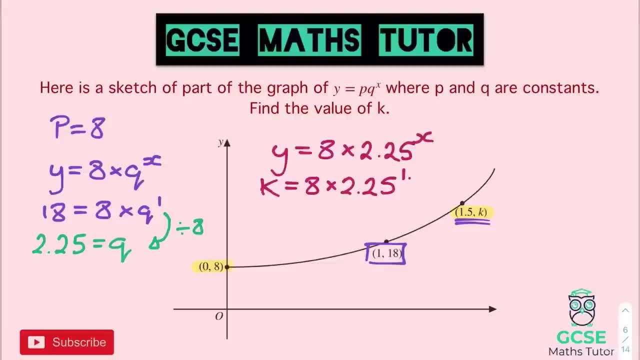 of 1.. So the power of our x value 1.5.. And again, all we need to do is type that into the calculator and we get a value 27.. And there we go, and there's our final answer. Let's just highlight. 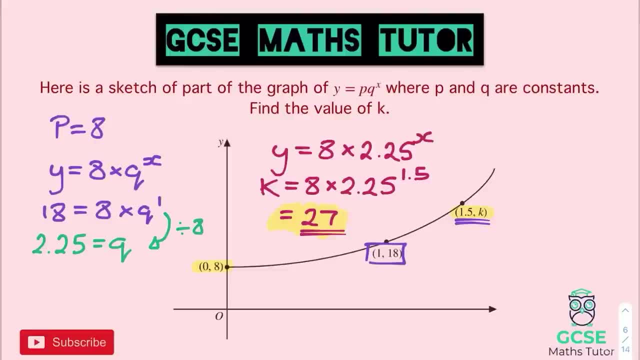 that, And there we are. our y coordinate in that case is 27.. So there we go. there is some work on exponential graphs, a few different types of questions there, but hopefully you found that useful and helpful And, if you did, please like.